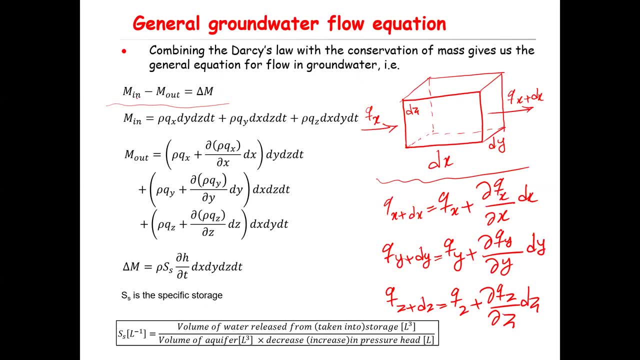 Here m in is the mass entering this control volume. the total mass entering this control volume minus the total mass exiting this control volume m out is equal to the change in the mass in this control volume. OK, so if you represent the velocity in the x direction by qx, 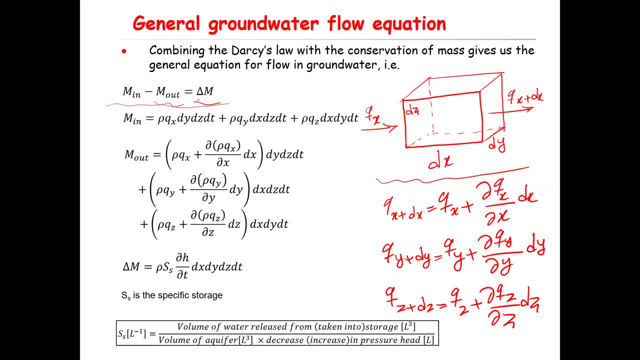 the velocity in the x direction on this side here will be equal to qx plus the derivative of qx with respect to x times dx. OK, and let's represent that by qx plus dx, And I didn't want to make this figure too crowded, but you can write the same equation here: 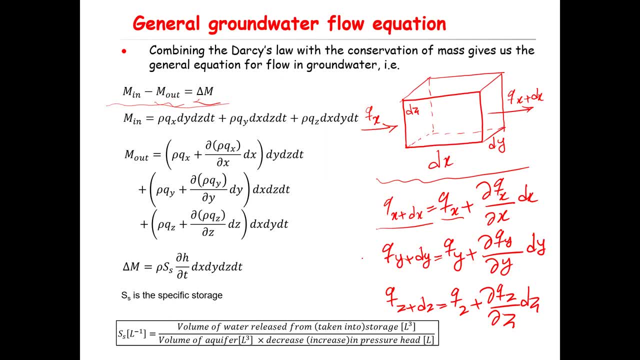 You can show the same velocity component for the y direction and for the z direction. So the velocity qy plus dy will be equal to qx. So the velocity qy, velocity in the y direction, plus the derivative of the velocity in the y direction with respect to y times dy. 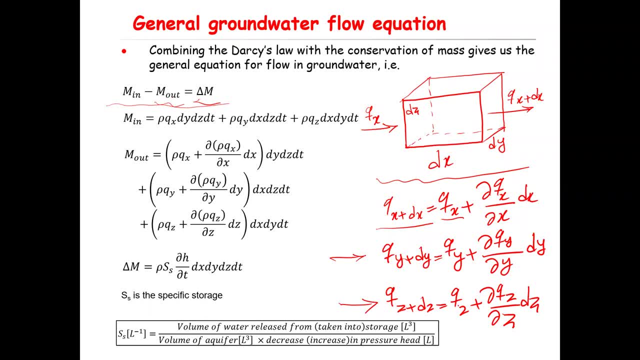 And the velocity qz plus dz in the z direction will be equal to the qz, qz plus the derivative of the qz with respect to z times dz. OK, and so in terms of the mass entering this control volume, you need to multiply this velocity that has the unit of length per time times the area. 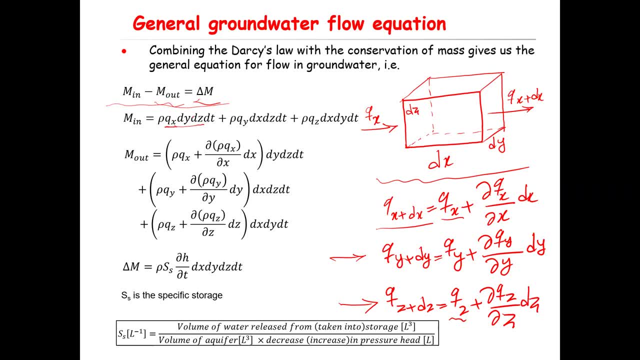 to give the volumetric flux, OK. and then you multiply that by density- OK- to get the mass flow rate. And then you multiply it by delta t or by dt to get the mass, That is, the mass entering this control volume in the x direction, from the x direction. 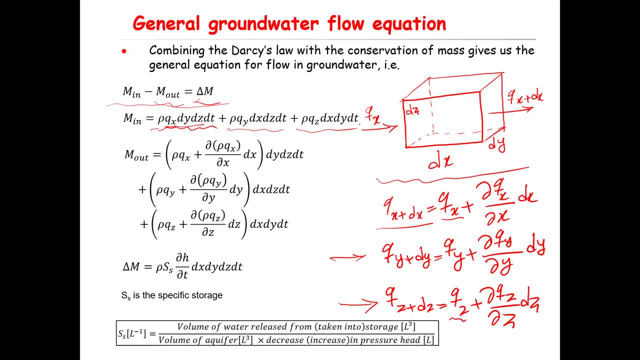 You can do the same for the y direction and for the z direction, And that is the m in. OK, You can do exactly the same for the m out. The only difference, The only difference here is, instead of qx, you basically use these three equations we wrote here: 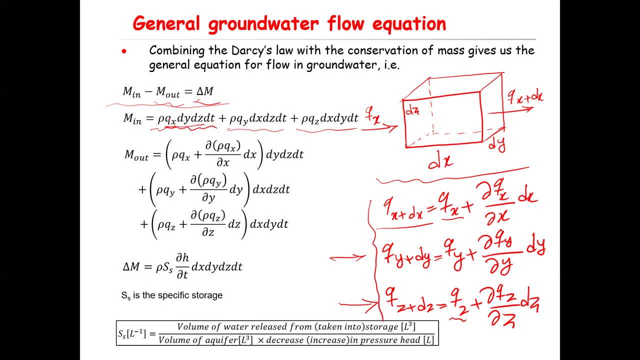 That is, instead of qx plus dx you need to write qx plus dx, But qx plus dx is equal to qx plus the derivative of the qx with respect to x times dx. OK, and if you plug these definitions of the velocity into this equation, you get m out. 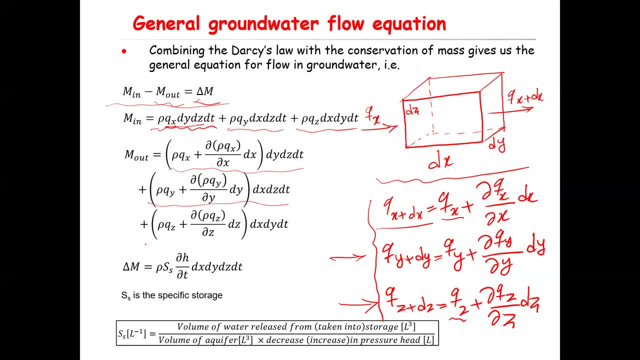 That will be equal to. that is for the x direction, y direction and z direction. So you have this. You have now an equation for m in, You have an equation for m out And also for delta m, the change in the mass in that control volume. you can easily show that that is equal to the density times, the specific storage ss that we had in the previous lecture, the definition of ss times, the derivative of the pressure head with respect to time times, the volume, that is dx. 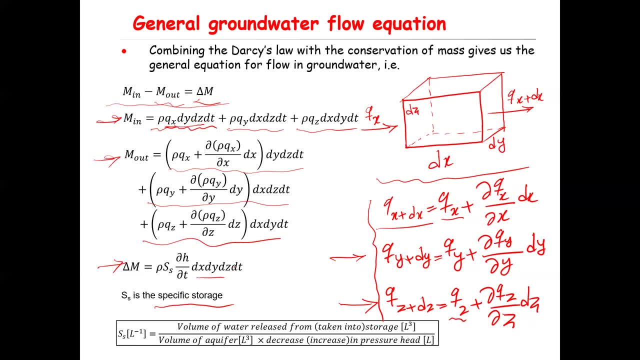 You can easily actually evaluate and see. this has the unit of mass, Because look here, ss is volume divided by volume times the decrease of the head right. So basically, if I Therefore, this one has the unit of one divided by legs. 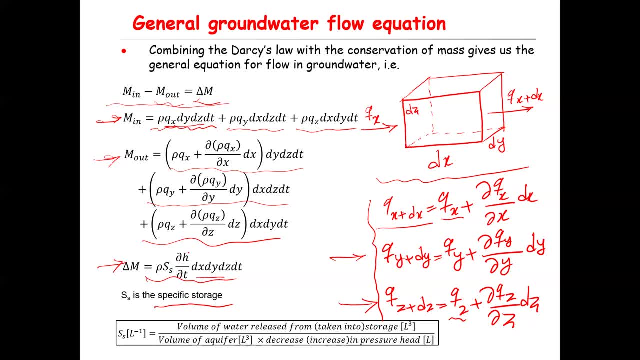 And if I multiply that by dh over dt, so the whole thing here will be will have the unit of one divided by time, And if I multiply it by this time, so the time will be will go out basically. So this term, this term- sorry, this term- and this term will be basically dimensionless. 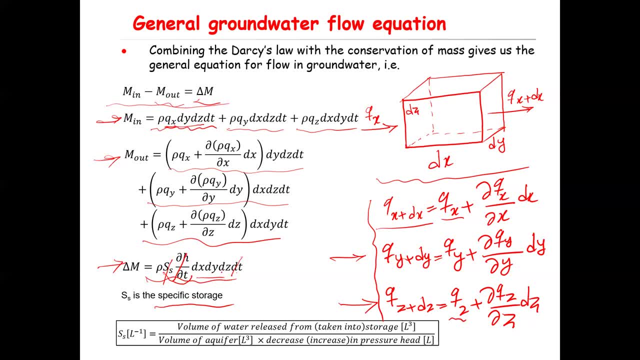 And then here you have dx divided by dz, that has the volume of the, the dimension of the volume times density. We know that that will be equal to the mass, So you can as well evaluate this equation like that, Anyway, so you have now an equation for m in. 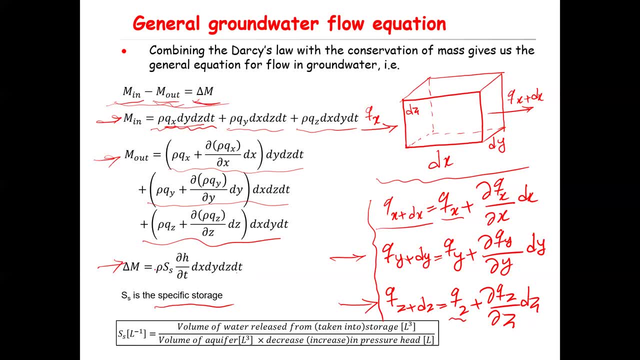 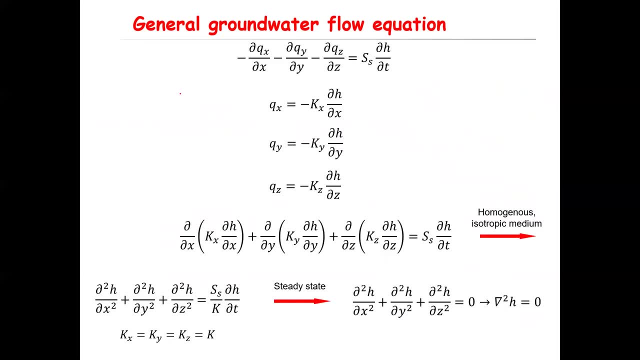 You have an equation for m out And you have an equation for delta m. Okay, If you plot this three term that we obtained here into this equation, you can show that minus derivative of qx with respect to x, minus derivative of qy with respect to y. 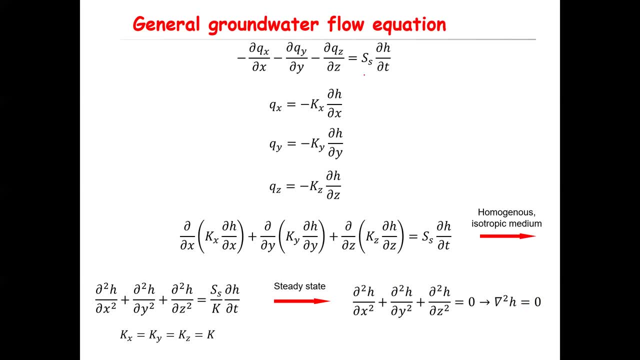 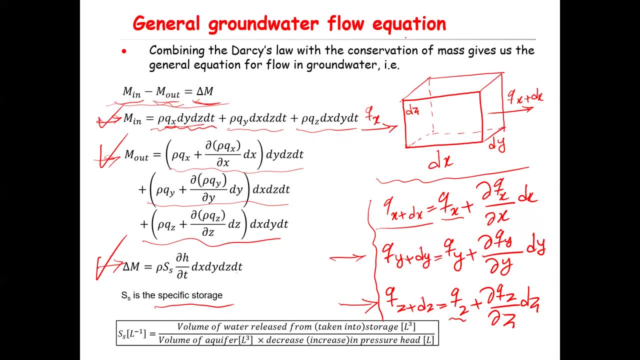 and minus. derivative of qz with respect to z is equal to ss. derivative of the pressure head with respect to time. Okay, That is very easy to calculate. Look here: If you write m in minus m out, this rho qx divided by dz, dt will be out by. 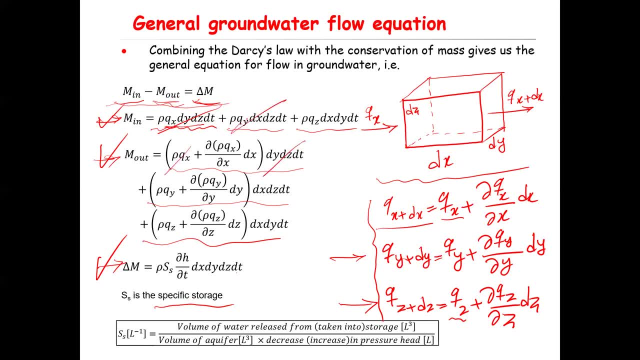 this rho qx divided by dz, dt, you see, and this one will be out by this term, and this one will be out by this term, And then, and then also the dx divided by dz will be out by this dx divided by dz, here and from the other side of the equation. 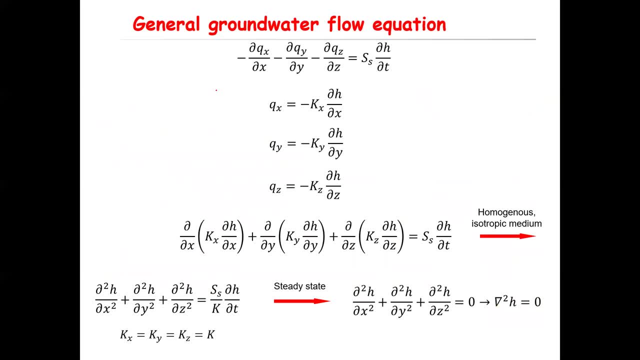 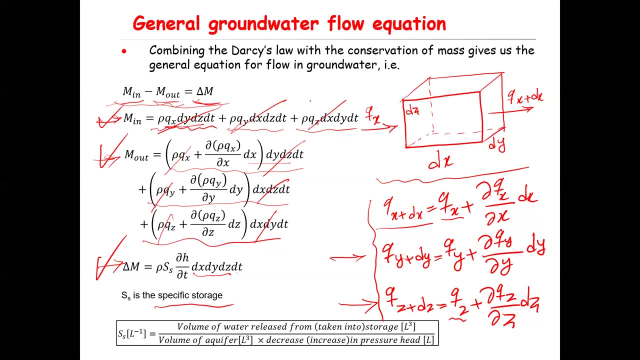 So it's a very simple algebra. You can easily derive this equation. And so now we have this equation here that is derived from the conservation of mass. Here for qx, qy, qz, we have Dorsey's law, So instead of qx let's write, by the way, here. you notice here that the density was inside this derivative. 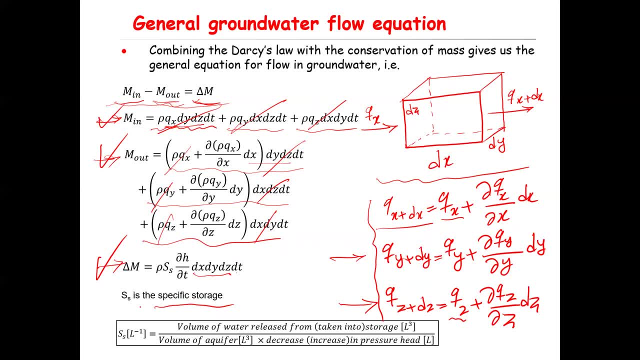 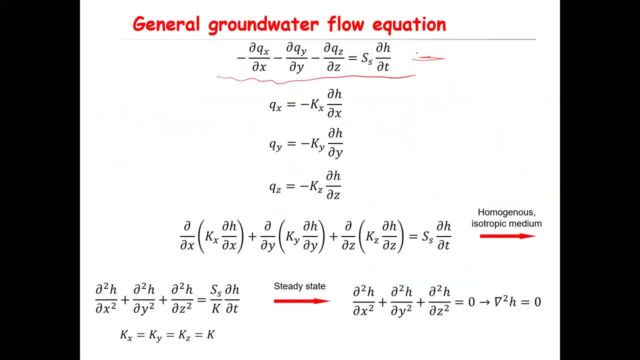 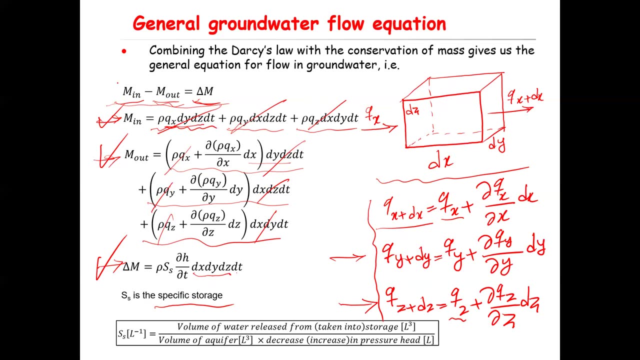 But now I take it out. In other words, you're assuming a density is constant, Okay, And that's why you don't see the density here in this equation. Okay, There's no density because you assume density is constant. And if you assume density is constant, so the rho, each of these terms, basically has density. 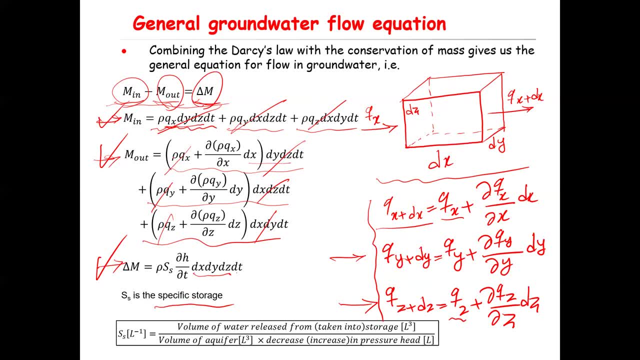 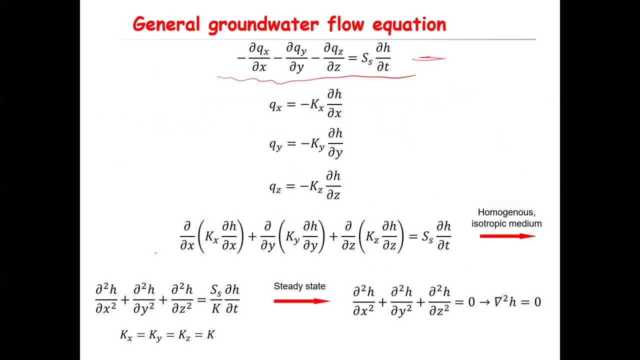 You see here, m in has the density, m out has density. delta m has density, The density basically cancels out from each side of the equation. Okay, Anyway, so instead of qx I write the minus kx derivative of h with respect to x, with respect to y, with respect to z. 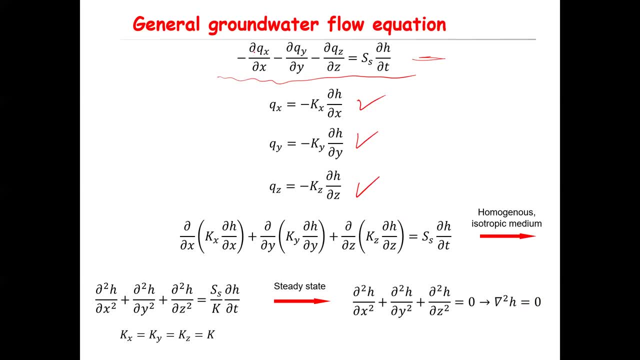 Okay, And then all I need to do now is just instead of: so that will be minus derivative of qx with respect to x Instead of qx, I write this equation. So minus times minus will be positive. So that will be derivative with respect to x, kx derivative with respect to. derivative of h with respect to x. here. 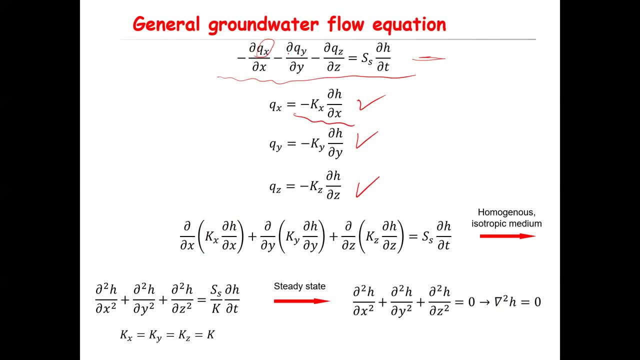 Okay, And then the same goes here. So I have rho the derivative with respect to y. it's here Instead of qy. I put this there. Okay, And minus by minus will be plus. The same here Again. derivative with respect to z is here. 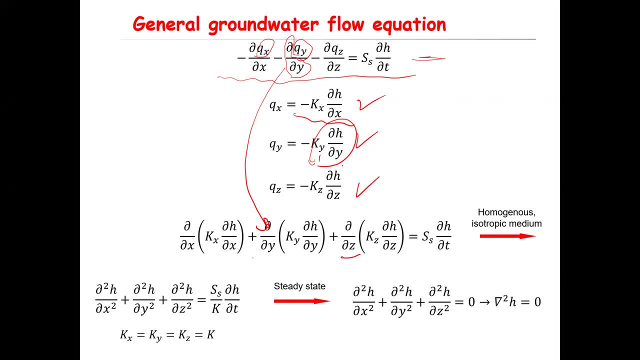 Instead of qz, I write kz. times derivative of h with respect to z: Okay, And that will be equal to s, So s times. the derivative of h with respect to time: Okay, h with respect to time. And then, if we assume, let me delete this one. 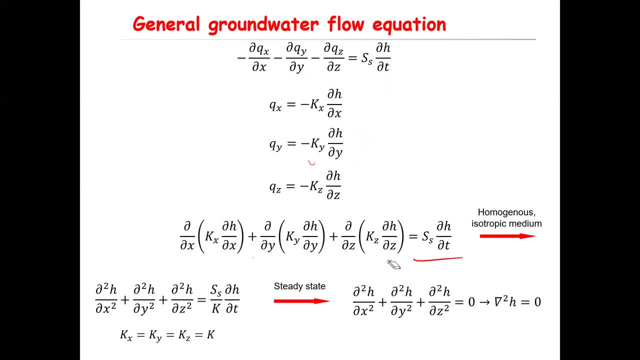 It's a bit crowded. So if we assume, if we assume the system, that my medium, my aquifer, is homogeneous, that means an isotropic, that means kx ky kz will be the same, And let's represent them by k. 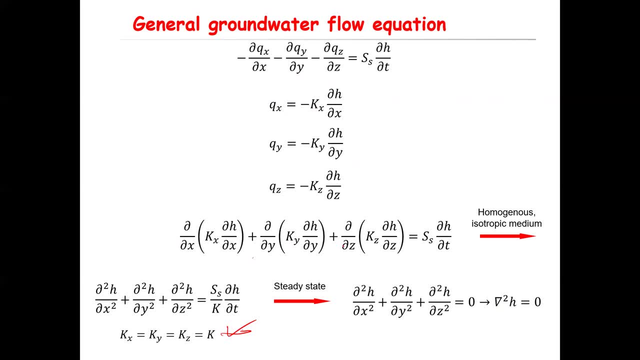 Okay. So therefore I can divide all terms here from each side of this equation, by the letter k, by the parameter k. Therefore, that will be the second derivative of h with respect to x2,. second derivative of h with respect to y2, second derivative of h with respect to z2 will be equal to ss divided by k, because I divided everything by k times. derivative of h with respect to time. 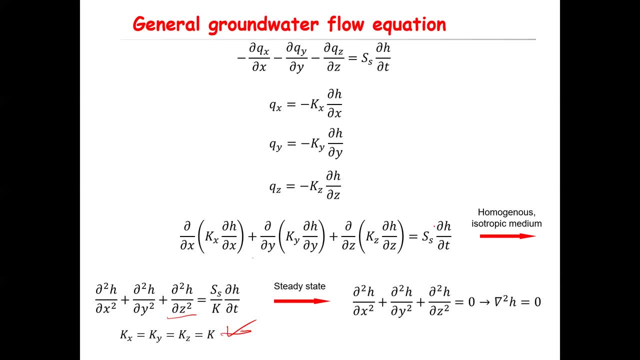 And then, if you assume you're dealing with a steady state condition, this term will be equal to zero. Therefore, the second derivative of h with respect to x2, plus the second derivative of h with respect to y2, plus the second derivative of h with respect to z2, will be equal to zero. 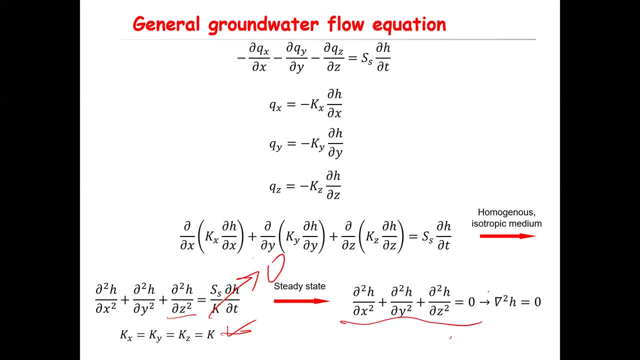 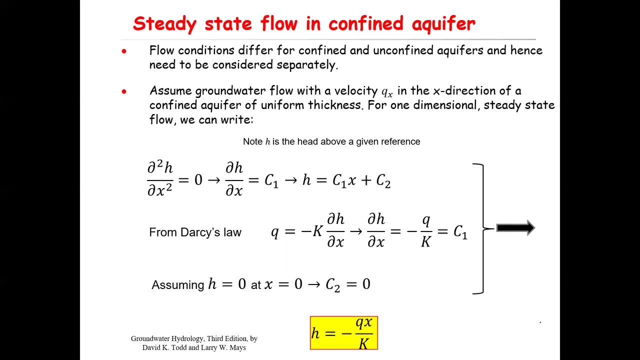 In other words, del square h will be equal to zero, And that is a beautiful equation that is used to describe the general flow in groundwater. Okay And yeah. So now we have this equation. The flow condition basically differs from confined and unconfined aquifers because you will have a different boundary condition, and you will see it in the next few minutes. 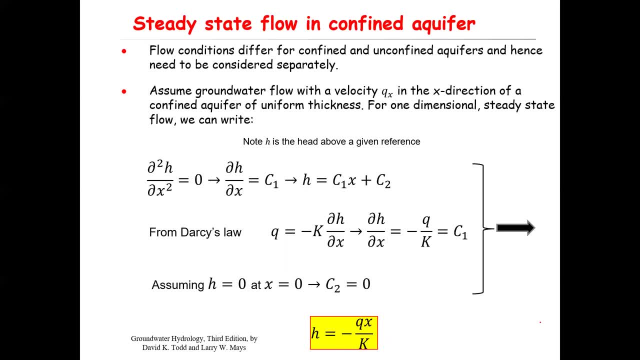 Okay, So we can now solve this equation for different boundary conditions. Okay, So let's first consider this case, That is, let's assume groundwater flow with a velocity qx in the x direction of a confined aquifer of uniform thickness. So that means I'm now solving this equation. the solution of this equation here. 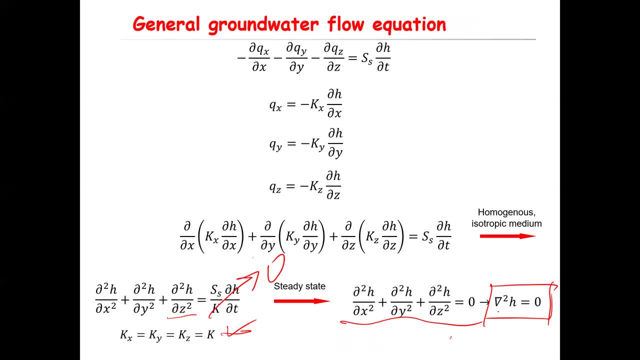 For confined aquifer and it's a 1D flow. Since it's a 1D flow only in the x direction, that means this will be equal to zero and that will be equal to zero. So you will have only the second derivative of h with respect to x2.. 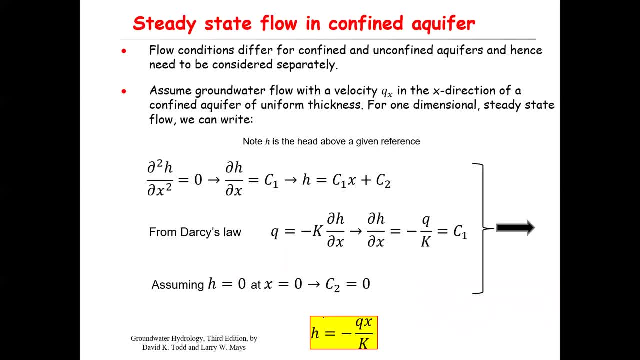 Sorry, the second derivative of h with respect to x will be equal to zero. Okay, So the second derivative of h with respect to x will be equal to zero. Okay, So we are dealing with a confined aquifer and the flow in the x direction. 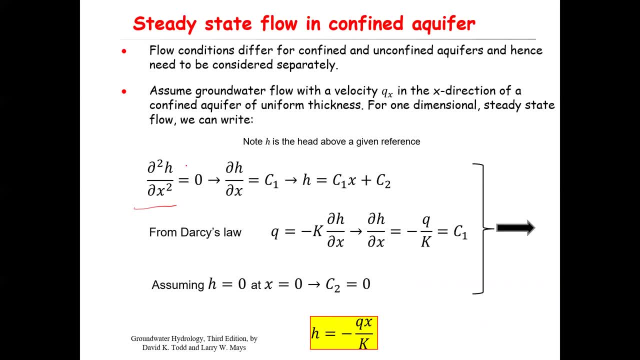 Therefore this is an easy interview. Therefore we can conclude here that the derivative of h with respect to x should be a constant. And you can take one more derivative, one more integral here. That will be the parameter. h here will be equal to c1 times x plus c2.. 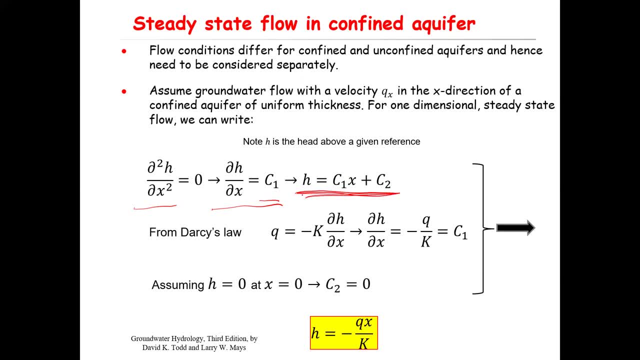 Okay, But obviously you need to calculate the constant of the integral here, That is, c1 and c2.. So from Dorsey's law we know that q, the velocity, is equal to minus k times the derivative of h with respect to x. 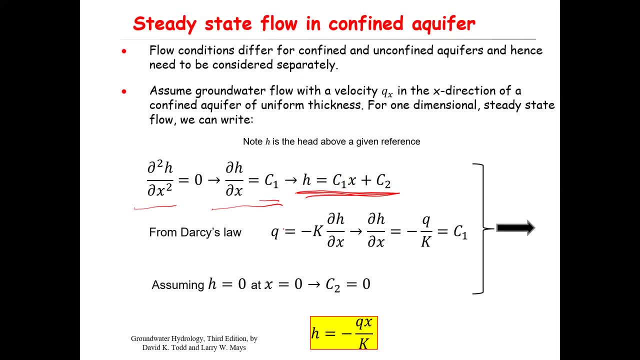 In other words, the derivative of h with respect to x is equal to minus q divided by k. That is from Dorsey's law. And then when you look at this equation, if you take the derivative of h with respect to x, the answer will be c1. 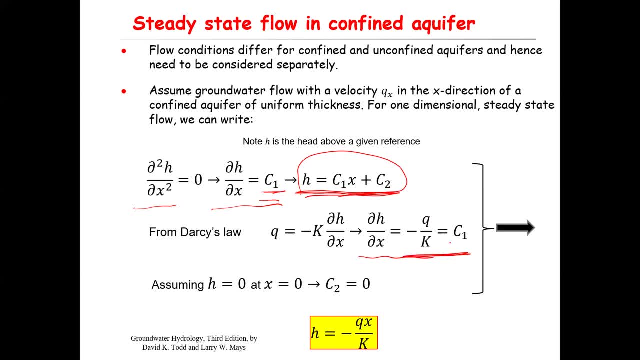 So, in other words, minus q divided by k should be equal to c1.. So that you already have that one. And also for the second constant of the integral c2, we just assume At x equal to zero, the h is equal to zero. 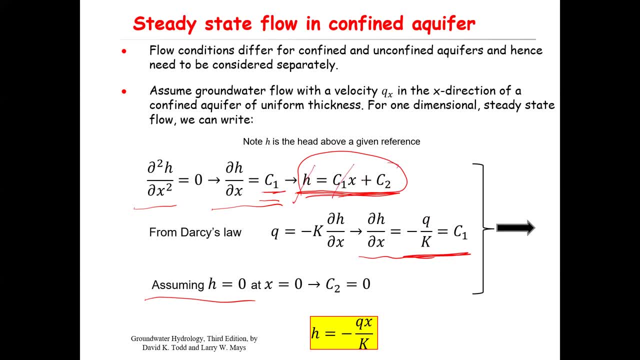 And if you put here x equal to zero, h equal to zero, that means c2 will be equal to zero. c2 will be equal to zero here And so now I have this parameter, c1.. I have the c2.. I plug these two into this equation. 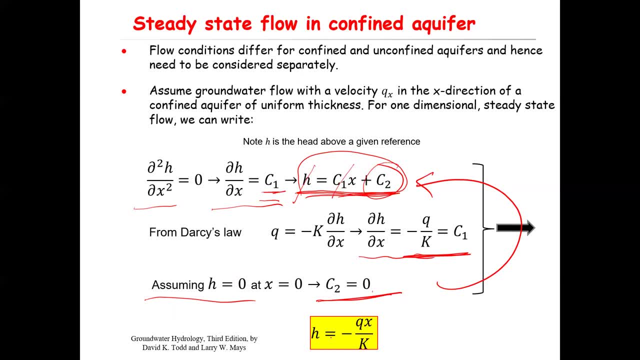 Therefore, you can show that h, that is the head, is equal to minus q, That is the velocity times x, That is the distance divided by k. Okay And so, yeah, that is the, That is the flow equation for confined aquifer. when you have 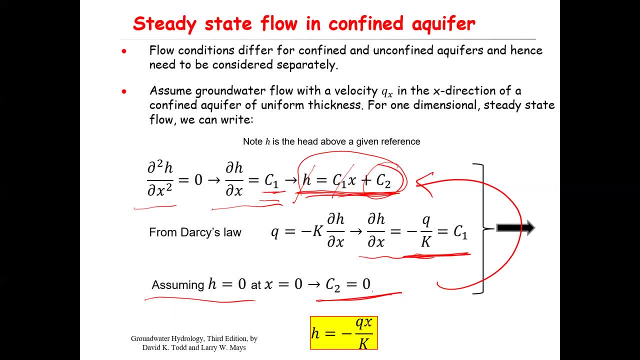 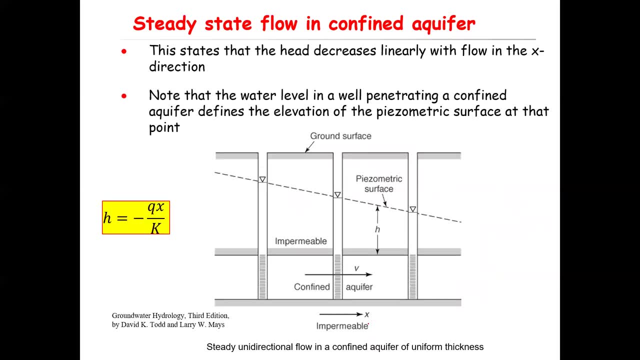 When you're dealing with the, When the aquifer has a uniform thickness, and also you're dealing with the 1D, flow in the x direction. Okay, So So let me read it from here: This states that the head decreases linearly with flow in the x direction. 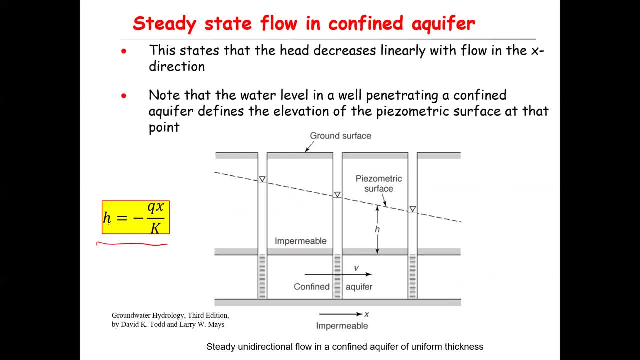 As you can see here, if you plot this line, you see it's a linear line. If you plot h with As a Versus x, you see it will be a linear line, with the slope of Minus q divided by k. 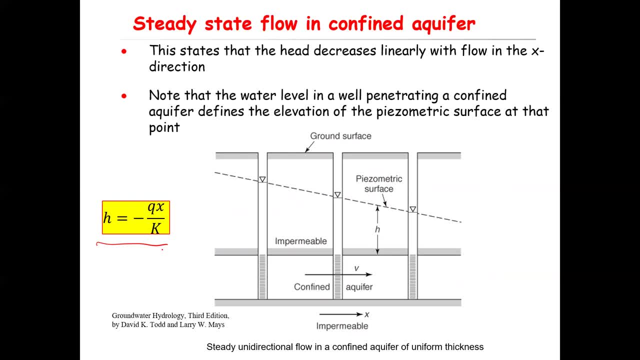 And, yeah, in the x direction, the head is decreasing linearly. Note that the Yeah. so here, actually, this picture is a. So this is, You're dealing with a confined aquifer. I say it is confined because it is confined by two impermeable layers. 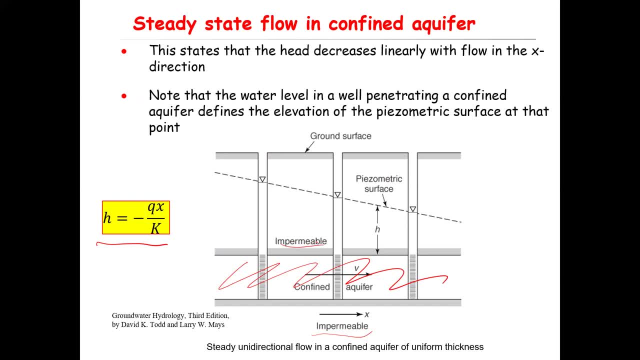 As you can see here, this is impermeable from top, from bottom and from top Right, And then the head here is a straight line And if the flow is in this direction, the head here linearly decreases, as with the flow in the x direction. 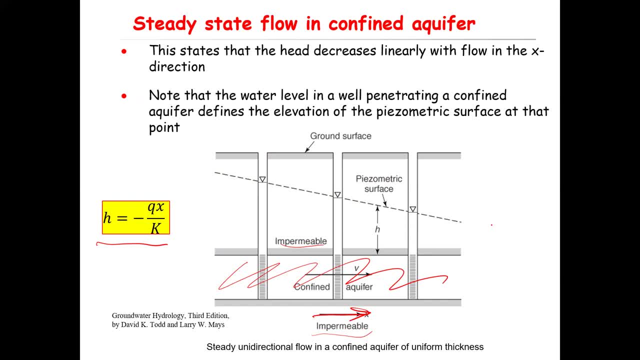 Okay, And if you remember, in the previous lectures we defined what is the piezometric surface That is not at the water level in a well penetrating, a confined aquifer. Here you see, here this is a well penetrating, this confined aquifer. 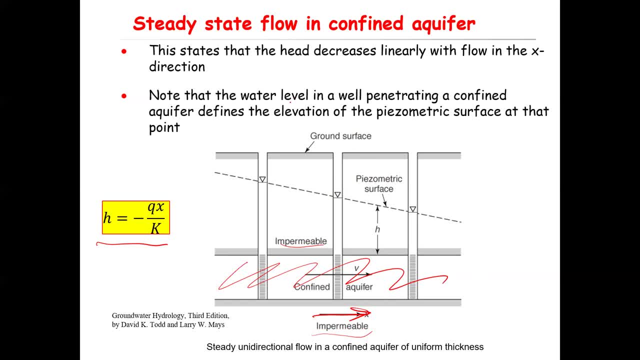 The water level in a well penetrating a confined aquifer defines the elevation of the piezometric surface at that point. Okay, So that is basically the The head in that particular point. Okay, So here this one. this is the piezometric. 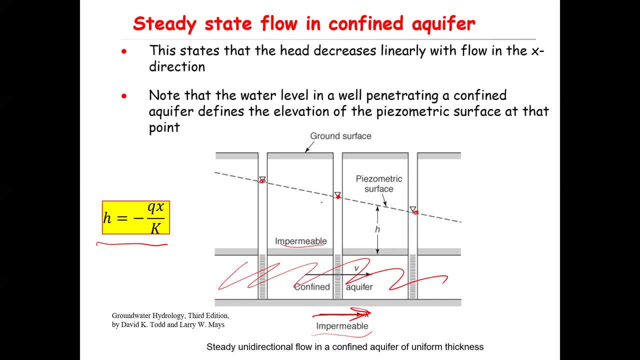 And the head. this is the piezometric head- And you connect them to each other. This gives you the piezometric surface. We had defined that in one of the previous lectures, Anyway. so that is the equation for the flow. 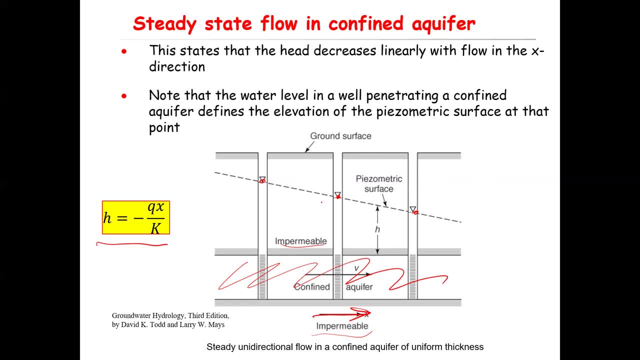 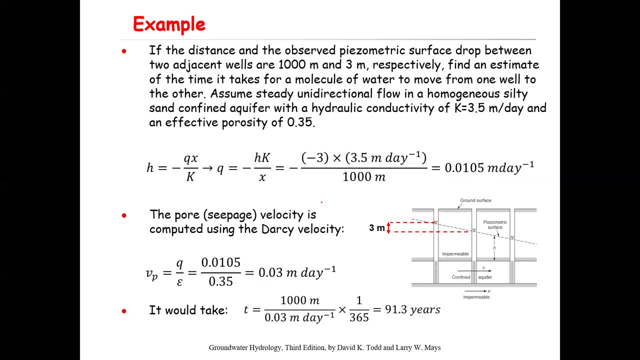 1D flow in confined aquifer with constant thickness. Okay, So there's an example here. This is quite a straightforward example, So let's solve it together. That is, if the distance and the observed piezometric surface drop between two adjacent wells are 1,000 and 3 meters respectively. 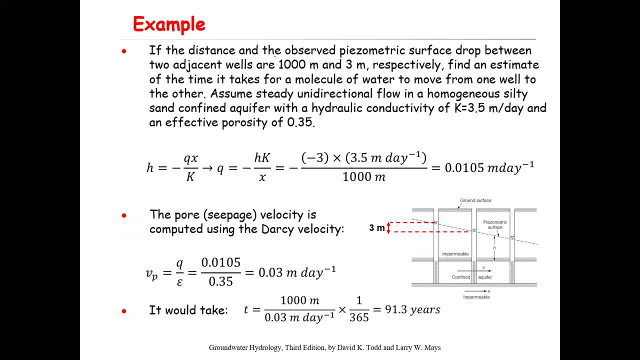 So you have two wells that are 1,000 meters away from each other And the drop in the piezometric surface is 3 meters. Okay, That's the question. So basically here let's say this is the first well here. 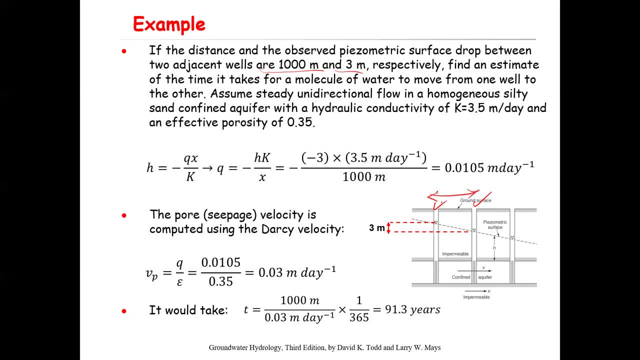 And I have the second well. The distance between these two well is 1,000 meters And the piezometric surface drops 3 meters, as you can see in this picture. So what's the question? Find an estimate of the time it takes for a molecule of water to move from one well to the other. 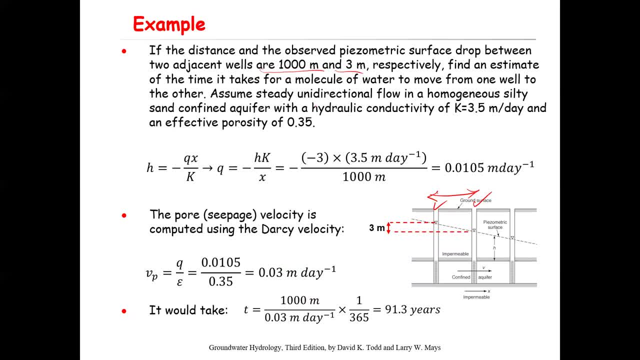 Okay, There are a couple of assumptions here. Assume a steady unidirectional flow in a homogeneous silty sand confined aquifer with a hydraulic conductivity of k equal to 3.5 meters per day and an effective porosity of 35 percent. 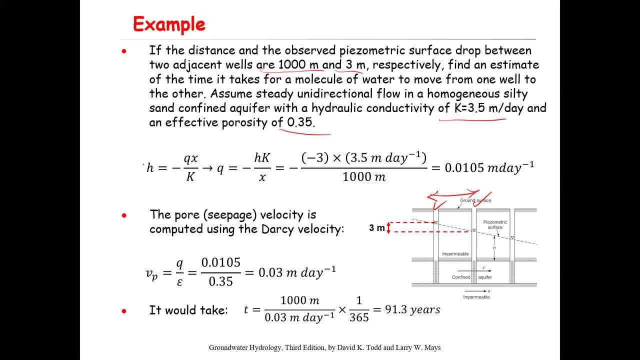 Okay, You just simply need to write down this equation that we just derived, that is, h is equal to minus q times x divided by k. Therefore, q, the velocity will be equal to h times k divided by x. And you have all these parameters. 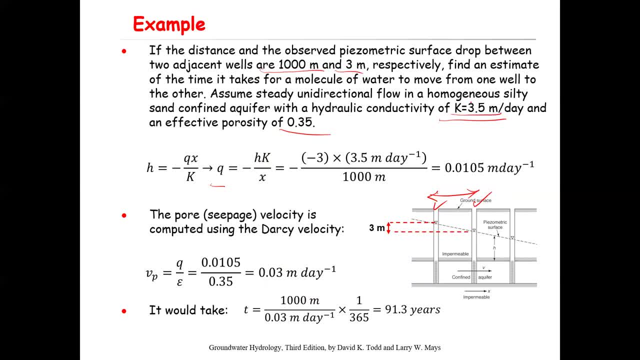 You have the h, that is 3 meters. You have the k, that is given in the question, 3.5 meters. x is 1,000 meters. And so you see, here, for h I put minus 3 because it is dropping right. 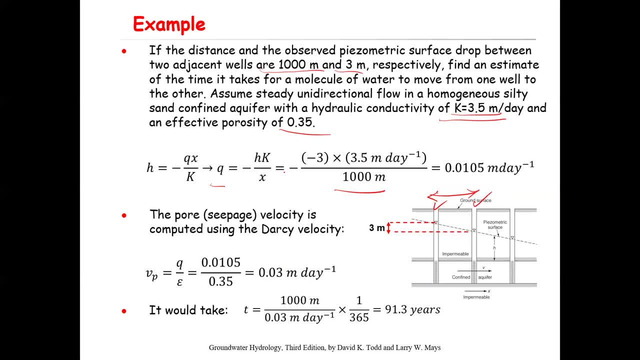 So that's why I put minus here. So minus times minus will be positive. So, anyway, the velocity, the Darcy velocity, will be this one. Okay, And if you remember, in one of the previous lectures I explained that to calculate the arrival time, 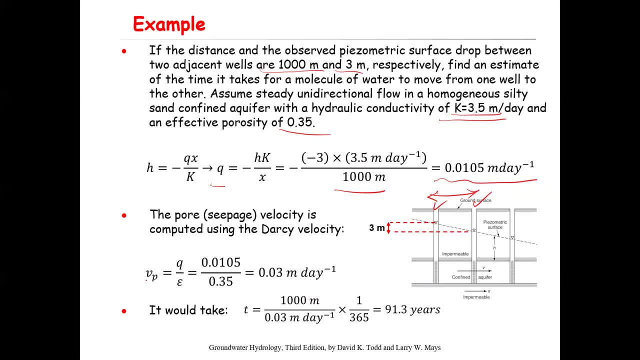 you need to work with the pore water velocity, And pore water velocity is equal to Darcy velocity divided by the porosity. And we do that because water only flows through the pore space. So you need to divide Darcy velocity, which is the average velocity. 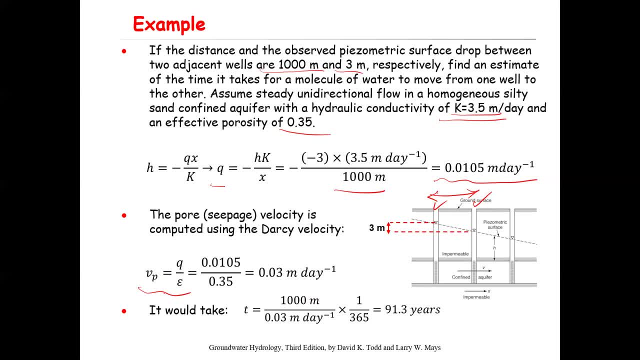 across the entire surface by the porosity to get the pore water velocity. And if you do that, so q is this one? You already put it here And the porosity was given in the question. That is 0.35.. 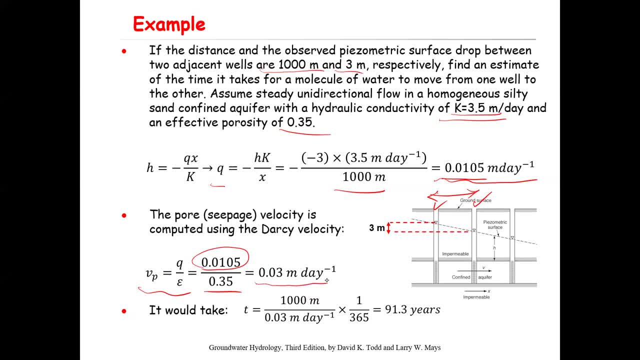 And that gives you the pore water velocity That is 0.03 meter per day. And the question was: how long does it take to travel this one kilometer distance? So from physics we know that the velocity is equal to length. 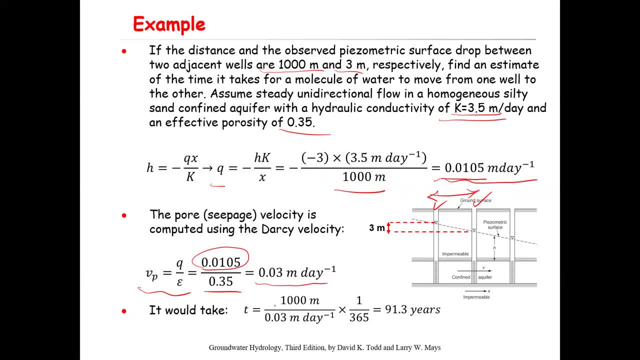 the distance divided by time. Therefore, time will be equal to the distance, That is, 1,000 meter, divided by velocity, which is 0.03.. And then I'm just expressing my answer in year. Therefore, I divide everything by 365, or multiply this by 1 divided by 365. 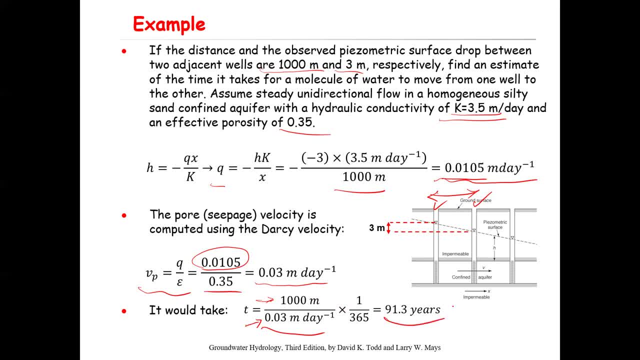 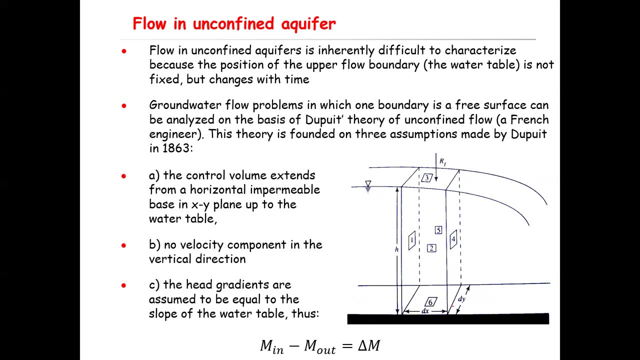 to convert the day to year And the answer will be 91.3 years. So it will take almost 91 years for the water molecule to move from one well to the other. OK, So that was the story about flow in confined aquifer. 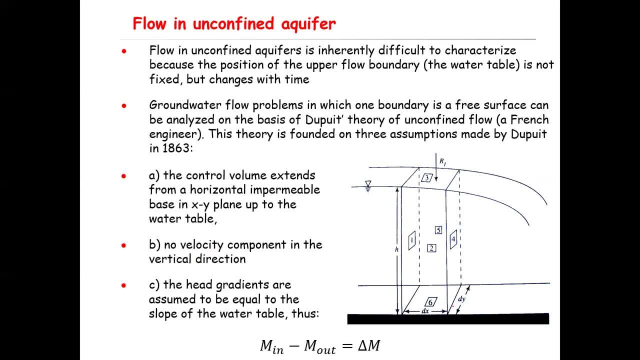 But of course you are as well sometimes dealing with unconfined aquifer. OK, So flow in unconfined aquifer is inherently difficult to characterize, because the position of the upper boundary layer, if the upper boundary or the water table, remember the unconfined aquifer at the top. 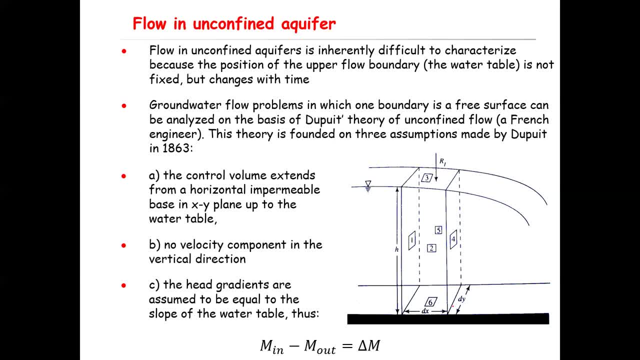 you had the water table That separates the saturated zone from the unsaturated zone, OK, And since that boundary or that water table is not fixed, so things are more difficult. with the unconfined aquifer, OK, And groundwater flow problems in which one boundary is a free surface can be. 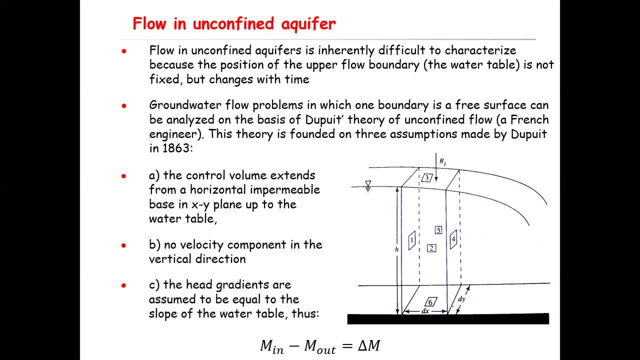 analyzed on the basis of DuPont theory of unconfined flow. OK, which was a French engineer, So he had three basically assumptions here And we will implement these assumptions in our analysis. That is A. the assumption is that the contour volume we consider extends. 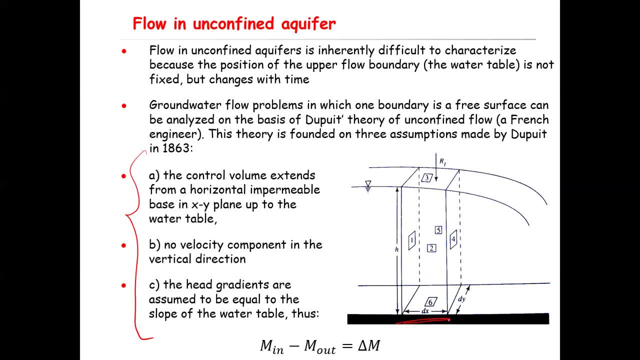 from a horizontal impermeable base like this one- the black base here- that's impermeable in the xy plane up to the water table. So that is this. If you remember, this sign indicates water table. So the contour volume extends from the horizontal impermeable base to the water. 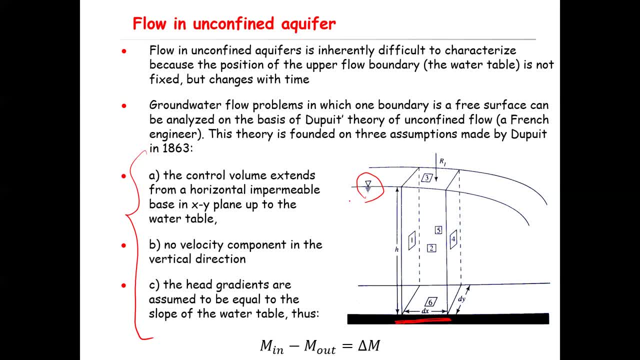 table. That's first assumption. The other assumption is that no velocity component in the vertical direction, So you don't have the qz anymore. So everything is in the horizontal direction. OK, That means you have qx and qy but not qz. 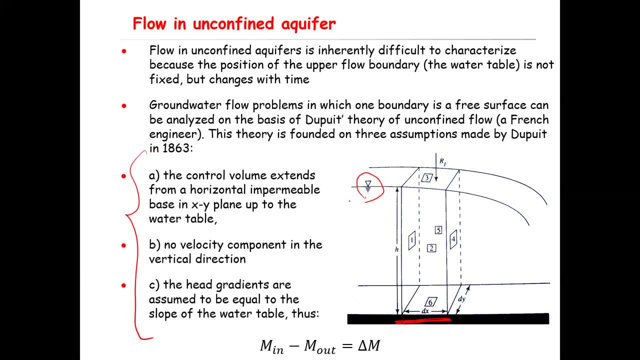 And also the head gradients are assumed to be equal to the slope of the water table. So you have these three assumptions, We are making these three assumptions. So now you can apply the conservation of mass again. That is mass in m in minus mass out is equal to delta m. 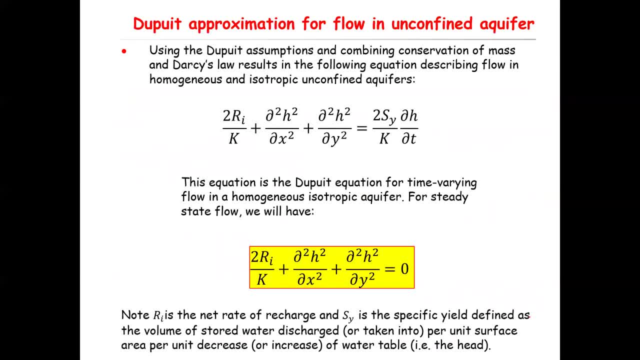 OK, I just present The final equation, So I don't go through the derivation. You can find this derivation almost in any hydrology textbook. OK, And I thought it's maybe not that necessary here to go through the derivation, So I'm just showing the final equation. 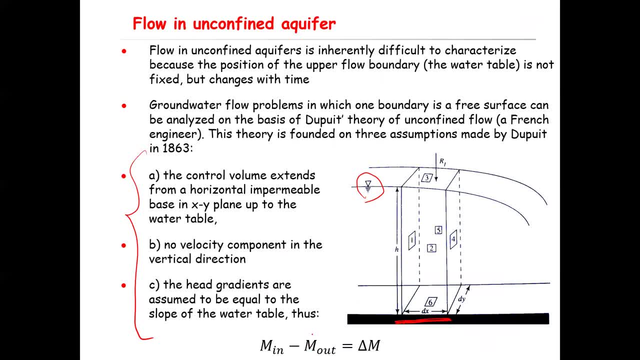 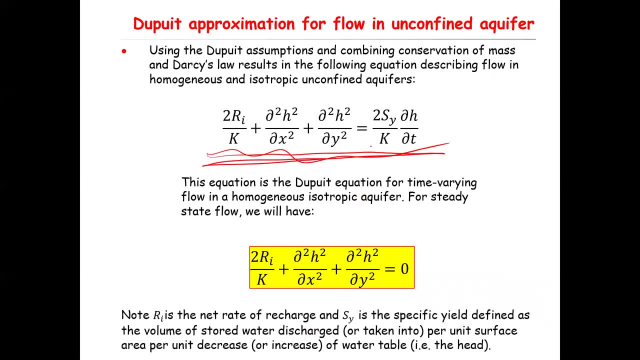 So, if you apply the conservation of mass and if you consider these three assumptions, you will end up with this equation, which is basically, again, the combination of the conservation of mass and Dorsey's law, which provides you an equation that can be used to describe flow in homogeneous and isotropic. 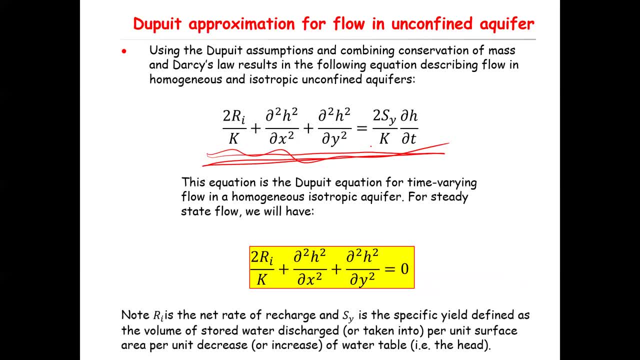 unconfined aquifers. OK, so that's the equation, This equation. you have two terms here. The rest is the same as before that you have the other parameters I meant. The k is the probability of hydraulic conductivity, H is the head. 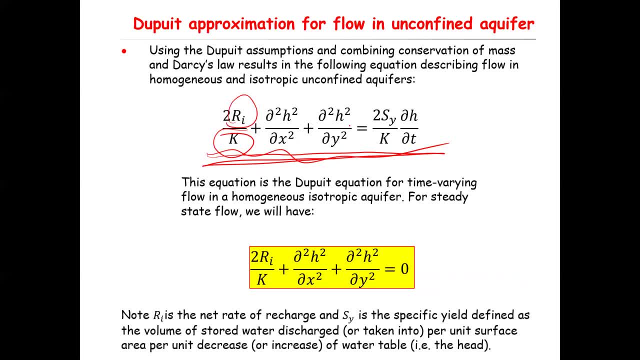 Pressure head And you have two new terms here, That is Ri and Sy. And Ri is the net rate of recharge OK to that aquifer. And Sy is the specific yield which we defined before in the previous lectures, in one of the previous lectures, as the volume of stored water discharged per 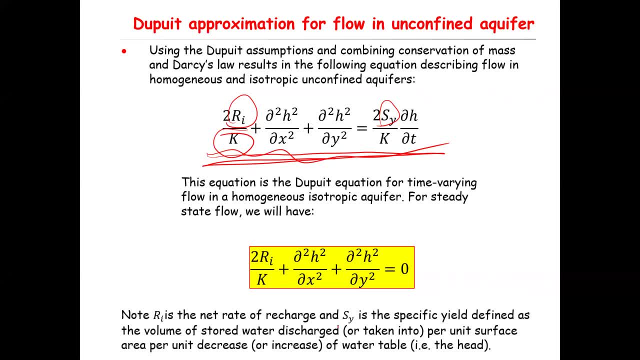 unit surface, per unit decrease of water table or per unit decrease of the head. OK, So you had this definition before. OK, So in the case of A steady state condition, in the case of a steady state condition like we did this, 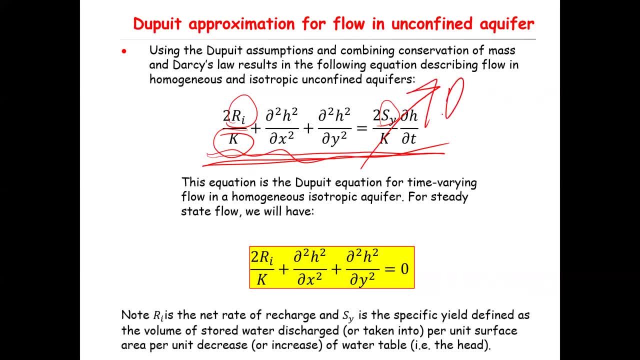 assumption in the past this term will be out, will be equal to zero. OK, So therefore, 2 Ri divided by k, that is, hydraulic conductivity, plus the second derivative of H with respect to x, plus the second derivative of H with respect to y. 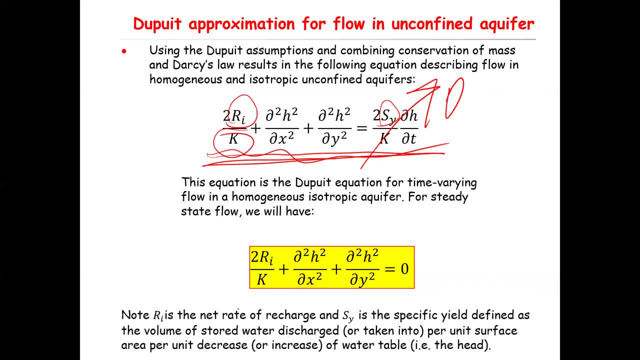 will be equal to. will be equal to zero. OK, And this is the equation That can be used to describe flow in homogeneous and isotropic unconfined aquifer under a steady state condition. OK, So. So now there's an example here. 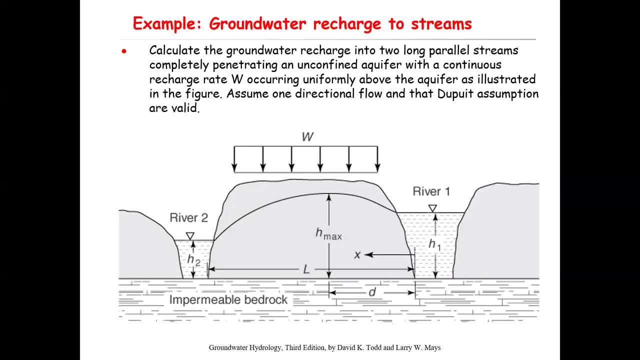 I wanted to go through the example so you will see how to apply this equation. The example is: calculate the groundwater recharge into two long parallel streams completely penetrating an unconfined aquifer with a continuous recharge, The continuous recharge rate W, occurring uniformly above the aquifer as illustrated. 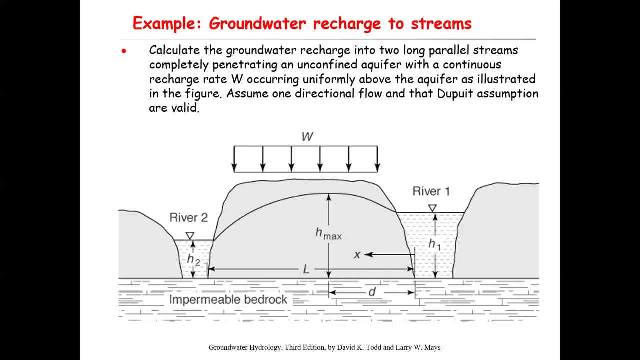 in the figure. Assume one directional flow and that two-point assumption are valid. OK, So these are the two rivers you have. OK, That's the cross-section. They are like flowing perpendicular to this screen And that is your aquifer here. 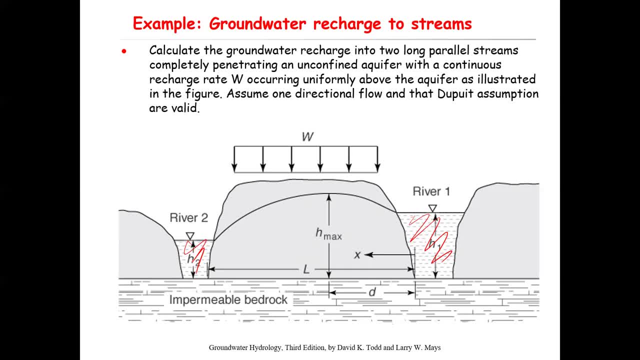 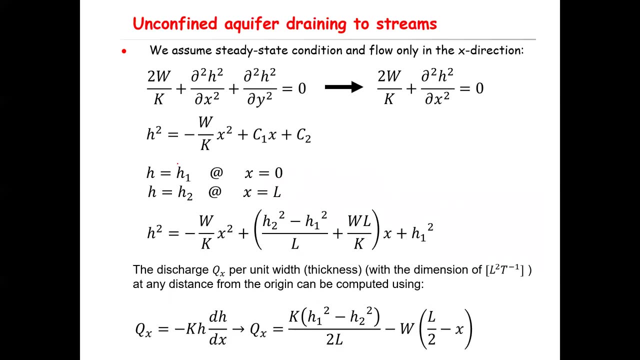 OK. So the question is: calculate the groundwater recharge into these two streams If, If you have this continuous recharge rate to the aquifer that is represented by W, OK, So to solve this example, you can literally just write down that equation that we just 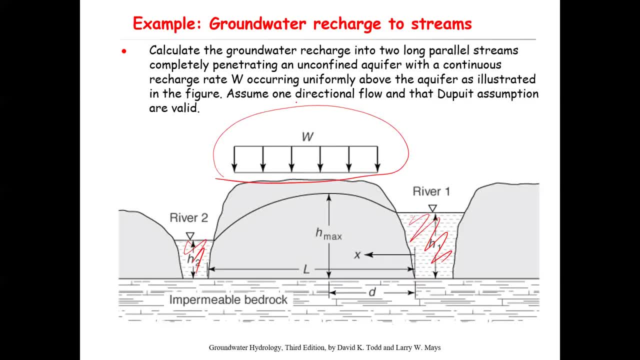 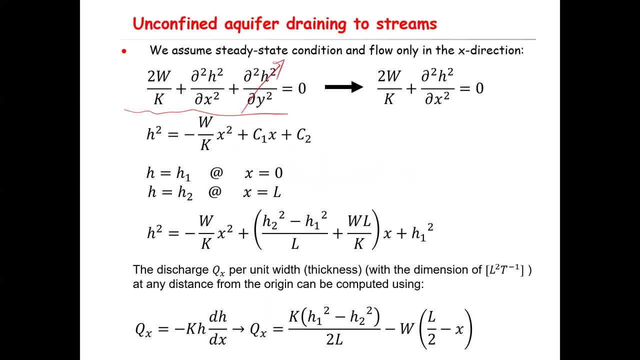 mentioned in the previous slide. Here the question says assumes one directional flow. So that means one term is out here. Let's say this is out. OK. So you will have only two. W divided by K, plus the second derivative Of H with respect to X will be equal to zero. 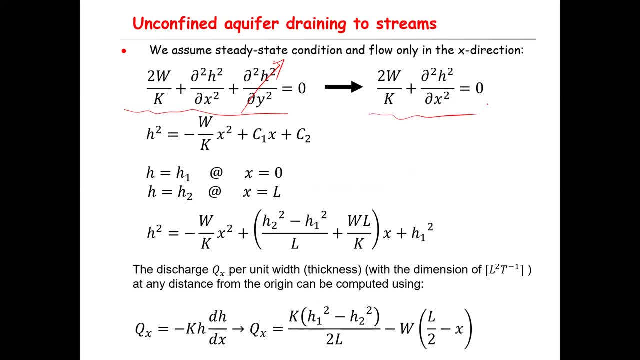 OK, And then you can easily calculate this differential equation And the answer will be: H2 will be equal to minus W divided by K times X2 plus C1, X plus C2.. OK, You just take this. take the integral of this equation two times. 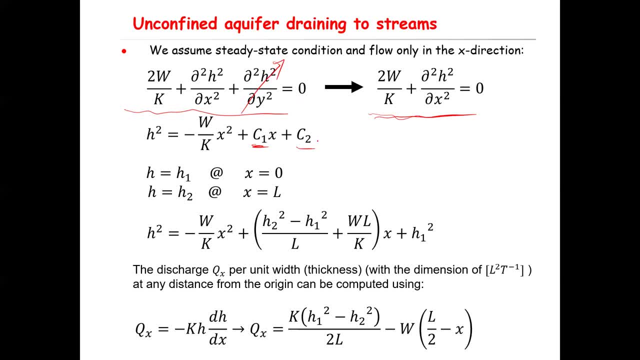 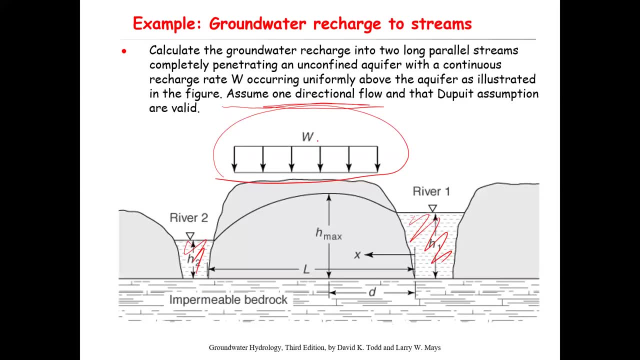 And then here you have two constant of the integral, C1 and C2.. So, but you have. the good news is you have the two boundary condition. that is here, Sorry, That is here, at X equal to zero, H is equal to H1, and at X equal to L, here and H is equal to H2.. 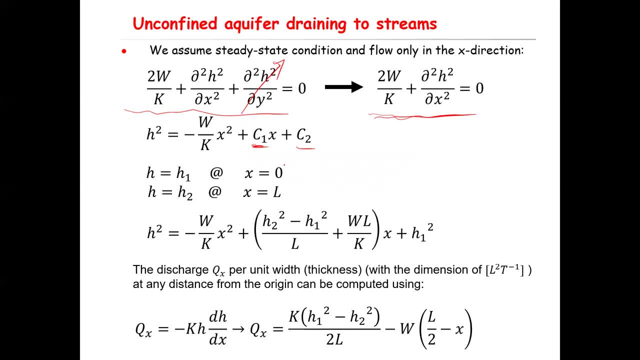 OK, So I have this two boundary condition: at X equal to zero, H is equal to H1. as at X equal to L, H is equal to H2.. And if I plug these two condition into this equation, then you can. you will have two equations. 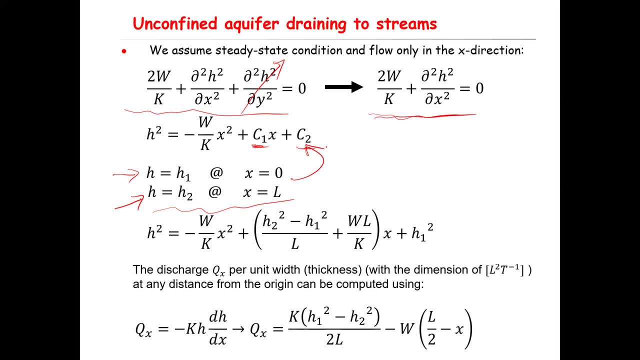 and two unknowns, Then you can calculate. You can calculate C1 and C2.. And if you plug it back to the same equation, you will arrive. you will obtain this equation, basically OK, That relates the pressure head, that yeah to the K and to the length and to the H1 and 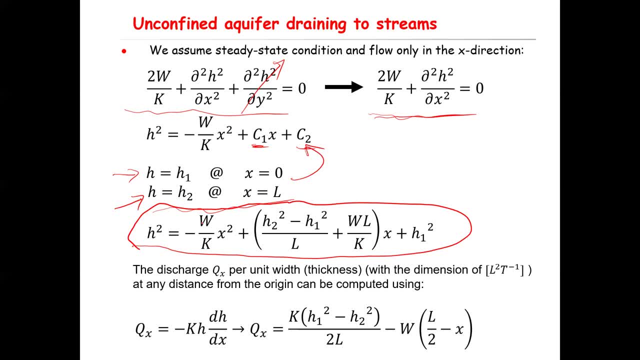 H2 and the recharge to the aquifer: OK, As a function of the, X from the, As a function of distance, X from the origin. OK, And sometimes as well the discharge QX per unit width or thickness at any distance, or. 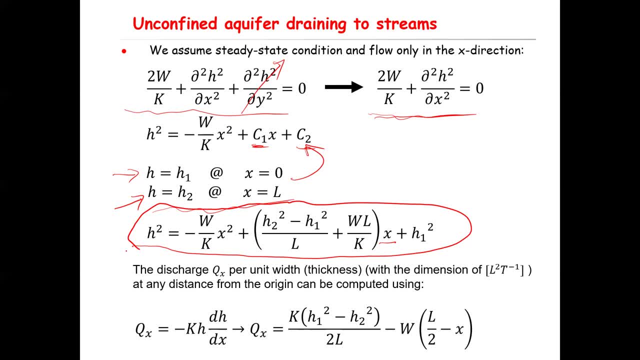 desire to calculate and that can be calculated by you. just multiply. basically, you have the Dorsey law. that is minus K, DH over DX. OK, That is the Dorsey's law. You multiply it by the H: OK, Because this is the discharge per unit width. 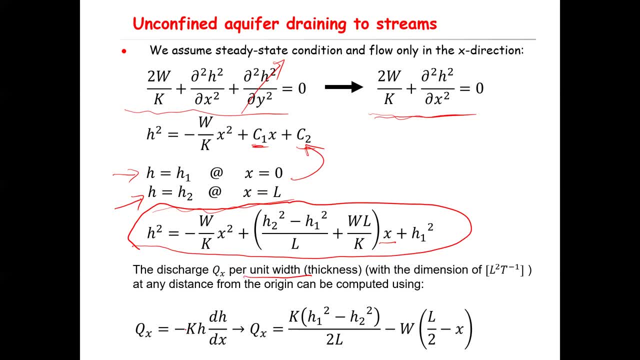 OK, And that's why- Because the Dorsey's law, The velocity has the unit of length per time. you multiply it by another length here. Therefore, the unit of this QX will be L squared per time. OK, So this is the discharge per unit width. 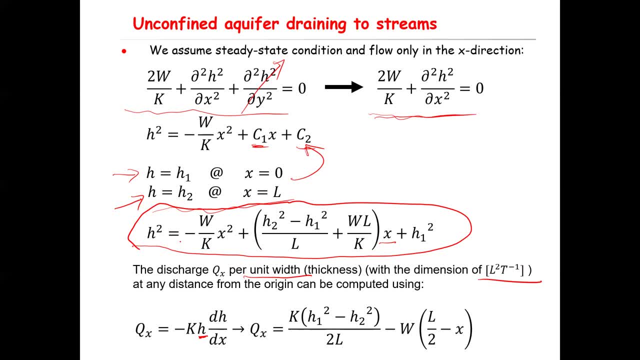 OK, And then. so DH over DX you can easily calculate by this equation. You have already the equation, and then you multiply it again by the H And if you do the mass, you will end up with this equation. OK, QX will be equal to this. 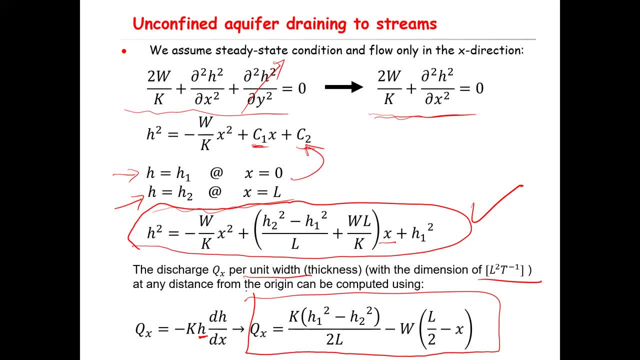 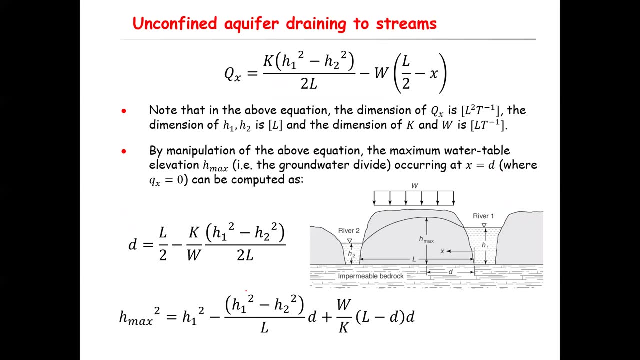 That is that. yeah, that relates the discharge per unit width to K, H1, H2, L and W at any given distance, X from the origin. OK, And then, but again, I just want to emphasize once again that in this equation, QX has the unit of L squared per time, and H1 and H2 has the unit of length and K and W. here they are. 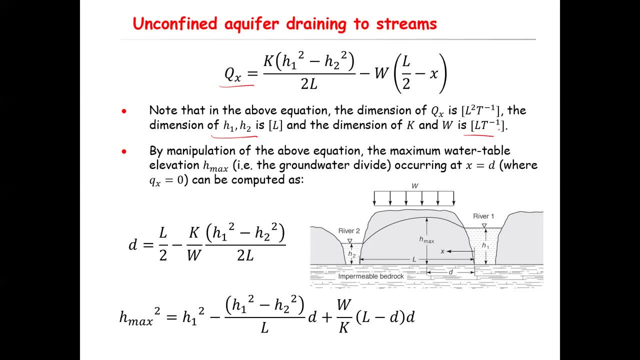 the, The K has the and W, they have the unit of length per time. OK, Also, sometimes as well, we wanted to know what is the maximum height of the maximum elevation of this water table, that H max here. as you can see, here that is called groundwater divide. 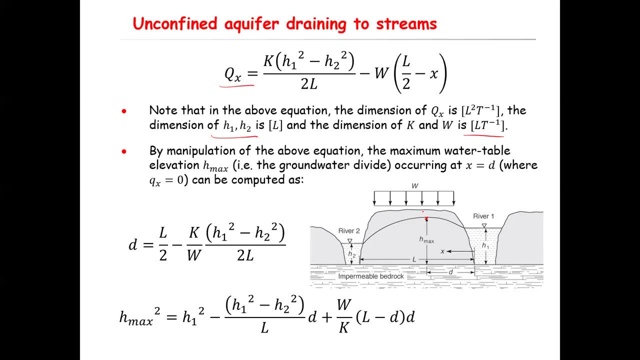 And also we wanted to know what's the location of that and to be using this equation. we can easily calculate that. basically, we know that at the maximum here the dh over dx is equal to zero, And from the Dorsey's law. so since Dorsey's law is the basic gradient of the head, 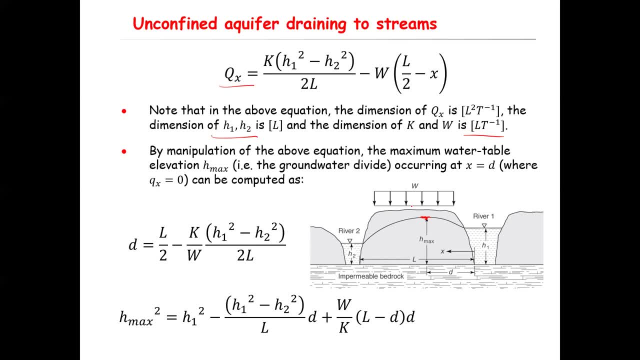 and since at that point the gradient of the head is equal to zero, that means velocity will be equal to zero. okay, So that means at that point qx is equal to zero. then you can rearrange this equation and calculate the x value at which qx will be equal to zero. okay, 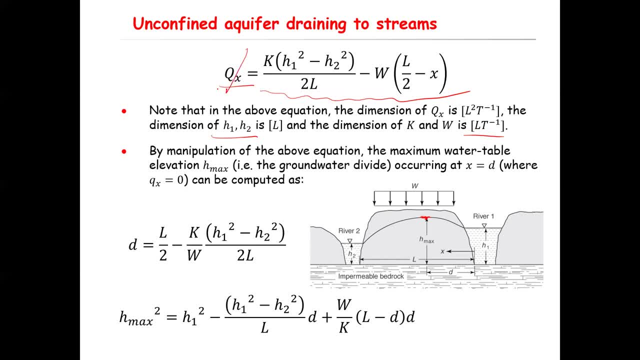 Because if this is equal to zero, all you need to do you need to divide everything by w here right, and bring the x to the other side of that equation. Then you will obtain this equation That gives that d here, as you can see in this picture here. 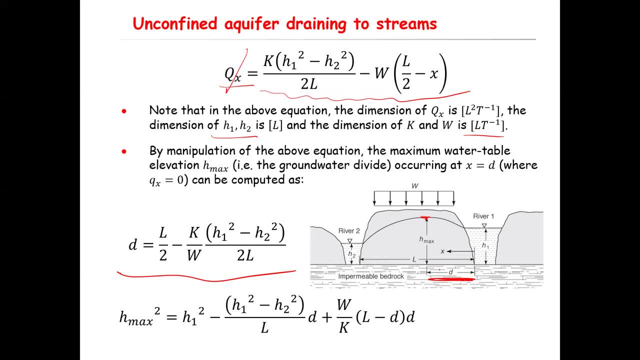 is the location at which the maximum water table elevation or groundwater divide occurs. okay, And then the value of the h max. now, since you have the, you have the d or you have the x value, you can plug it here in this equation. 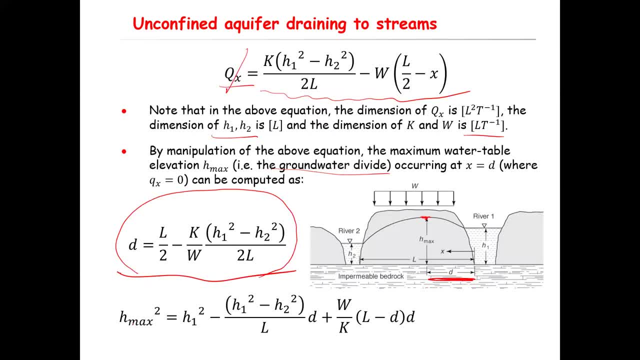 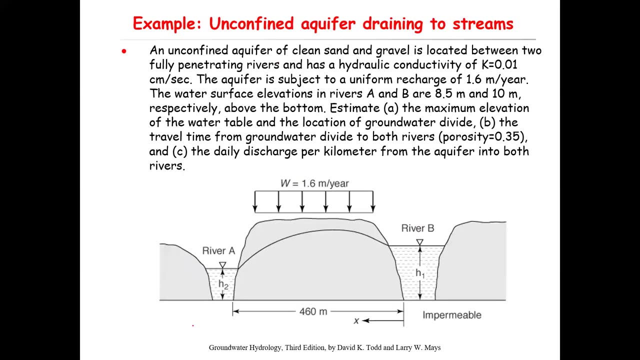 and then you can calculate the value of the h here, the maximum value, which will be equal to this one. So this is another useful equation, okay, Yeah, So there is an example here. I want to go through that example. It's very actually, just simply the application of this. 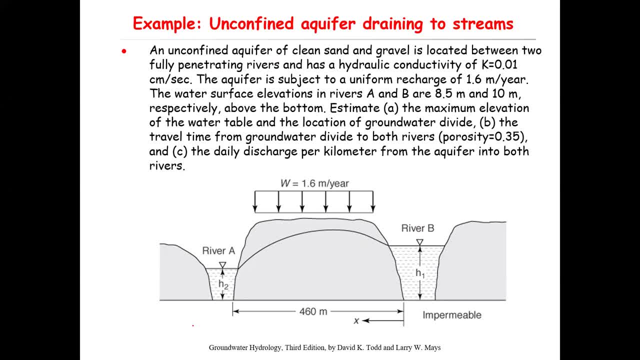 that simply shows you the application of the equations that we just derived. So that is an unconfined aquifer of clean sand and gravel, is located between two fully penetrating rivers and has a hydraulic conductivity of 0.01 centimeter per second. The aquifer is subject to a uniform recharge of 1.6 meter per year. 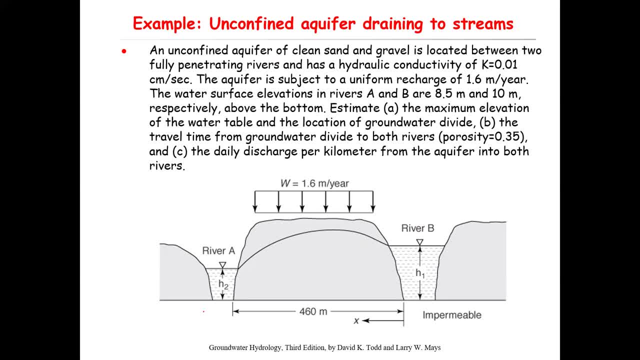 The water surface elevations in river A and B- so this is river A and this is river B- are eight and a half and 10 meters. So this is given. so h2 is equal to eight and a half and h1 is equal to 10 meter. okay, 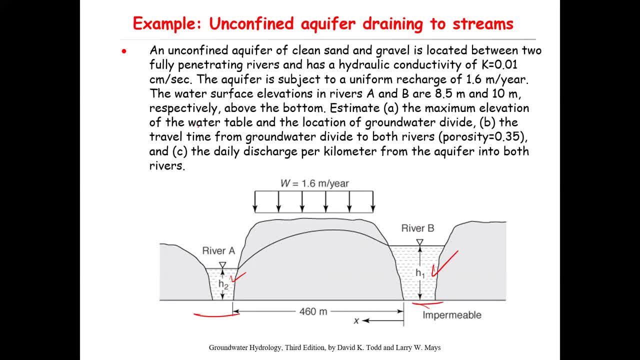 10 meter respectively above the bottom Estimate the maximum elevation of the water table. that is h max. So you have a question for that. and the location of the groundwater divide. Again, you have an equation for that. that is that B. 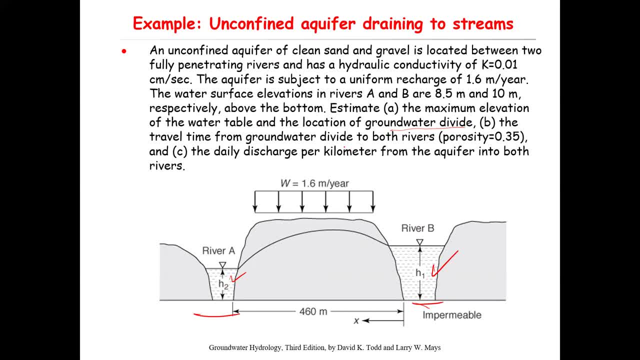 The second part of this question is the travel time from groundwater divide to both rivers. okay, So whenever there is a groundwater divide, let's say, for example, it's here if you calculate. so the question is: what's the travel time from here? 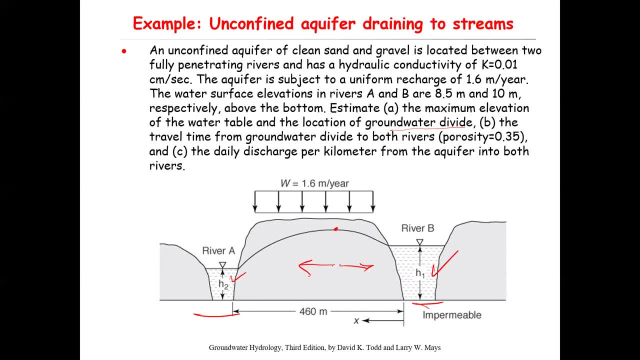 To river B or from here to river A. That's the second part of the question, assuming the porosity is 35%. And the third part of the question is the daily discharge per kilometer from the aquifer into both rivers. okay, 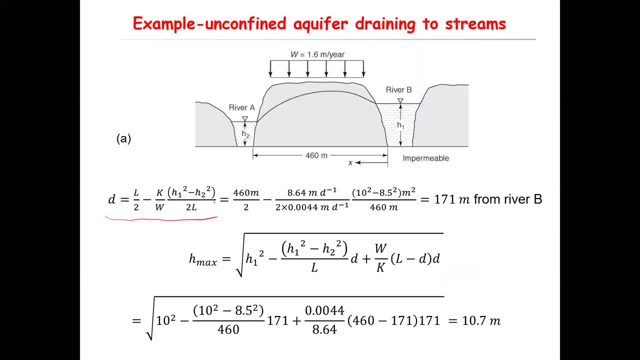 So so you just need to write down that equation we just derived to for the section A, that is, D is equal to this equation. So you have all the parameters here. The length is already given, that is 460 meter, and k is given in the question. 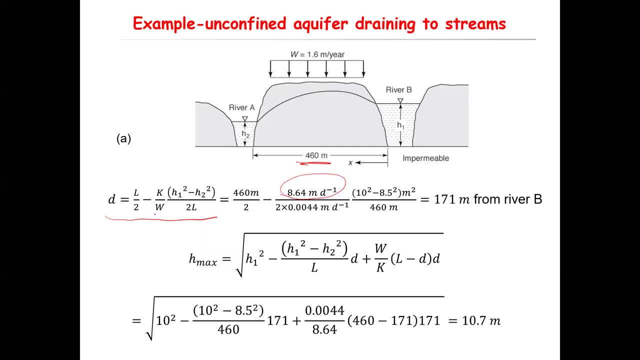 I just converted the unit to meters per day. okay, W the, the recharge rate has been given already. that is here. and then you have two and the two two is here. okay, There's one, two for this one and the other one is here. 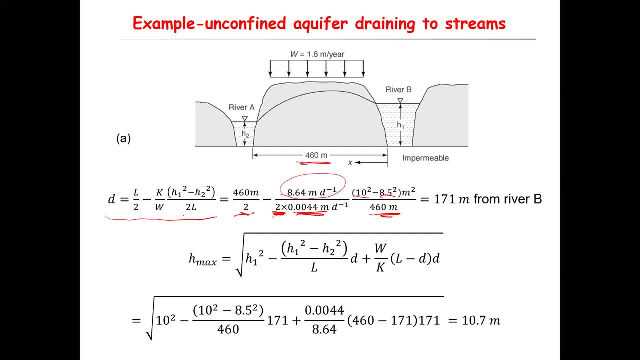 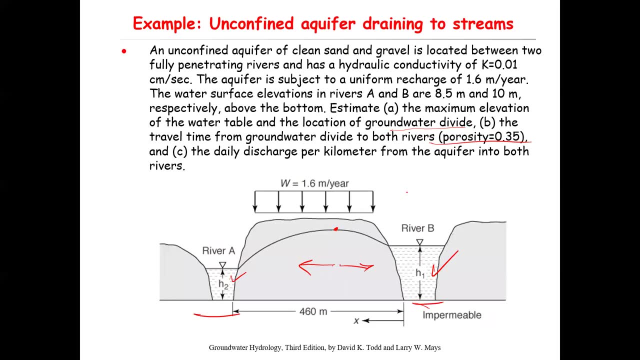 L already given, H1 given and H2 as well given. okay, Yeah, because H1, H2, yeah, that's correct, H1 and H2 was given 10 meter and 8 and a half meter okay. 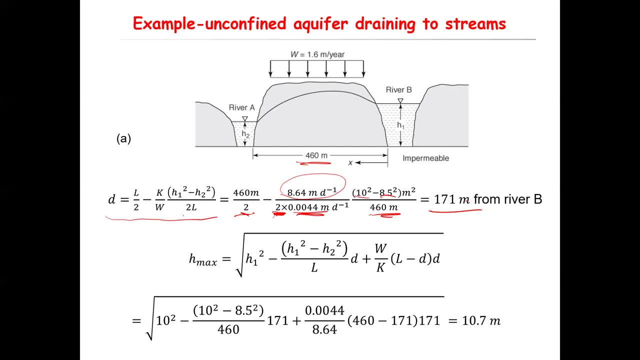 So if you do the algebra here, you you get 171 meter from river B. the X will be equal to 171 meter. okay, So that means if this is where the maximum occurs, this distance is equal to 171 meter from the origin. okay. 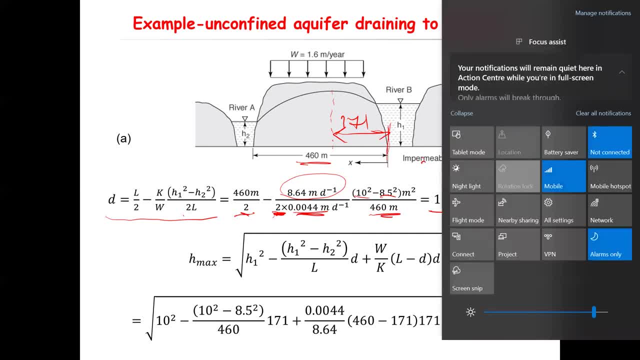 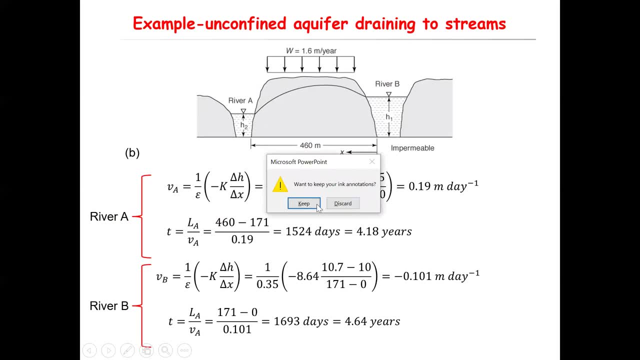 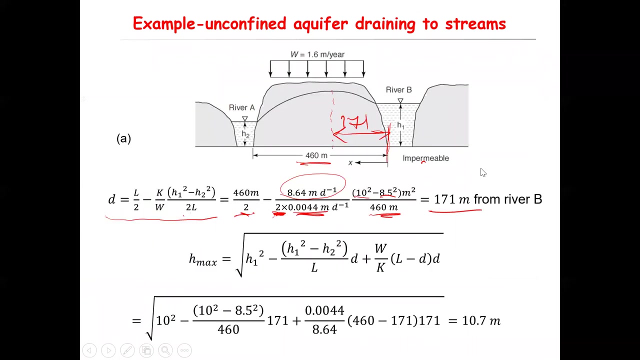 From the origin. Let me close this one, Sorry. Okay, perfect, Okay, perfect, Okay, perfect, I think yes, okay, so. so so we calculate the location of the H max. okay, So now the other part of section A was that: what's the maximum elevation of the water table? 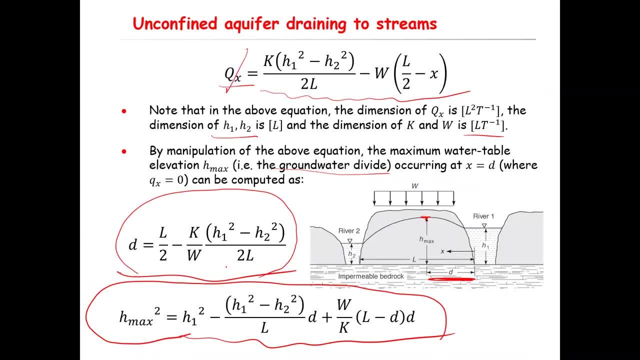 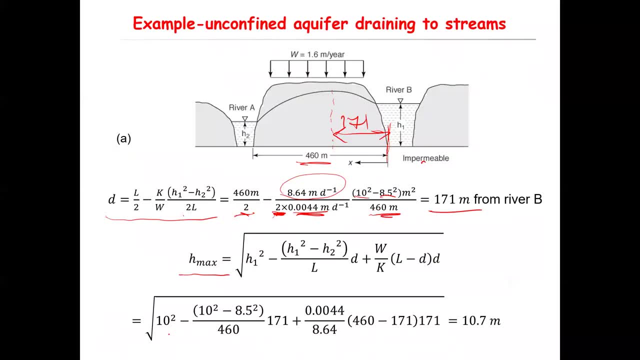 Again, we have an equation for that. as you can see here, this is the equation. So therefore, H max will be a square root of this side of the equation. okay, And that's literally okay, And that's literally what we're doing here. and again, you have all this parameter: H1, you have H2, you have D, you have you already calculated here. that is 171 meter W, given in the question K, given in the question L, given in the question. you just plug all the values here and you will see H max is it will be equal to 10.7 meter. okay. 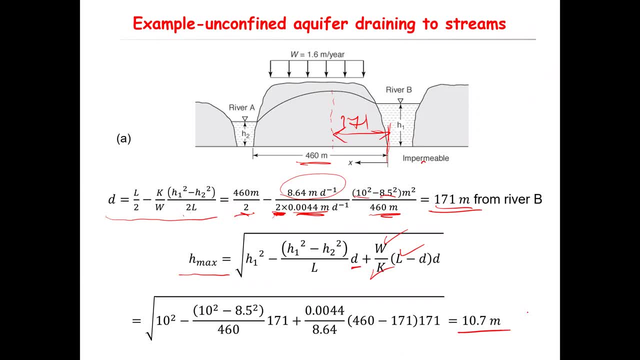 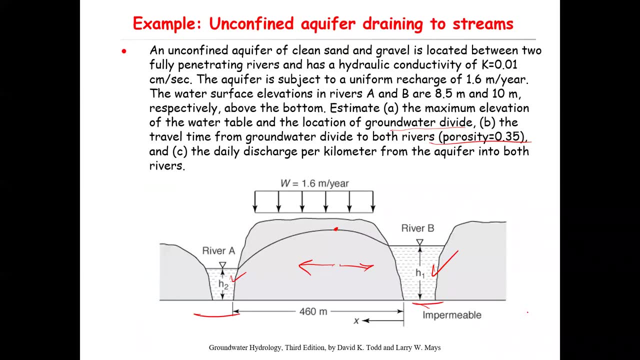 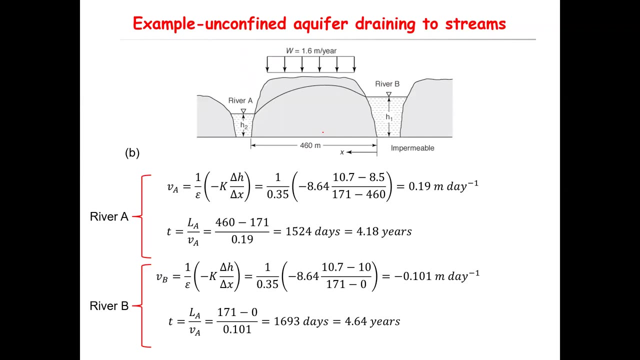 That's going to be the maximum elevation, okay, So the second part of this question was about what's the? basically, let's read the second part of the question. But the travel time from groundwater divide to the both rivers. so let's just calculate the time to river A. so first we need to calculate the pore water velocity, like the previous example, because travel time is about pore water velocity, and then you, knowing the distance, you can calculate the time. so this is the Darcy velocity, right? 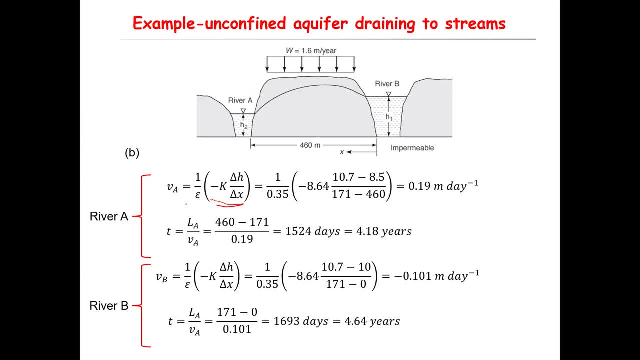 And I divide it by the porosity to get the pore water velocity. so the pore water velocity, therefore, will be equal to one divided by the porosity. that is given in the question times, minus K And K is equal to 8.64, that is again given in the question right times, delta H over delta X. so we are here and we just calculated this height is equal to 10.7 meter. 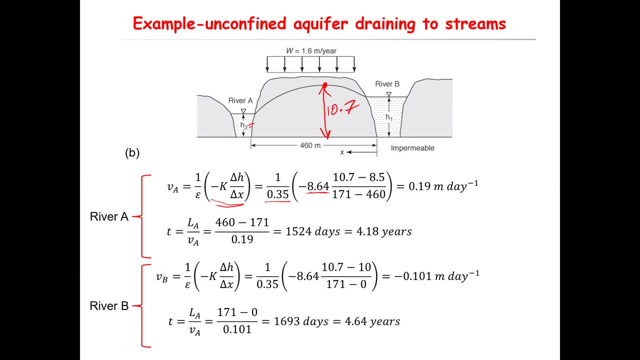 In the question, it's given that this height- H2, is equal to 8.5 meter and H1 is equal to 10 meter, and we know this distance is 171 meter. okay, So therefore W VA. 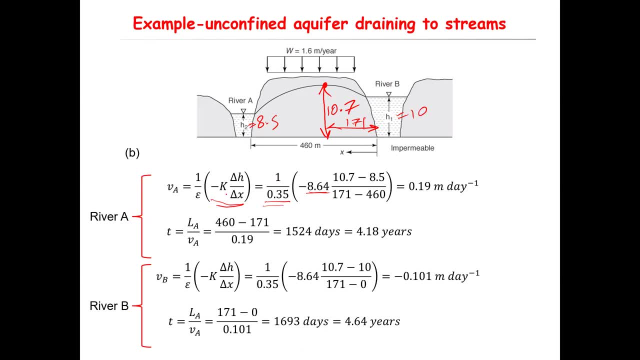 The pore water velocity toward A will be equal to one divided by porosity. times. K is given in the question, times delta H over delta X. delta H here 10.7, minus the H here 8.5,. divided by this, the X of this point minus X of that point. so X of this point is equal to 171, minus X of that point, that is 460. 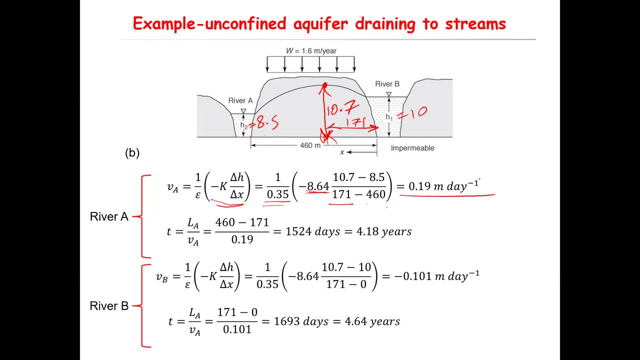 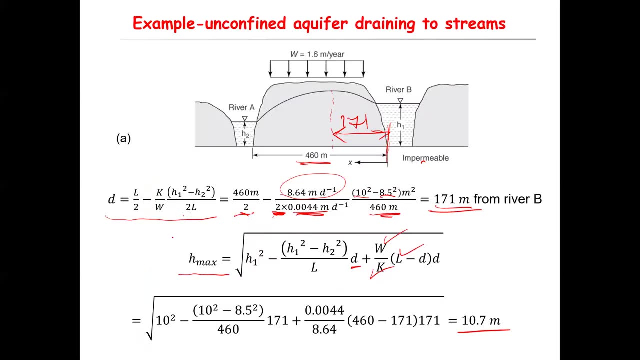 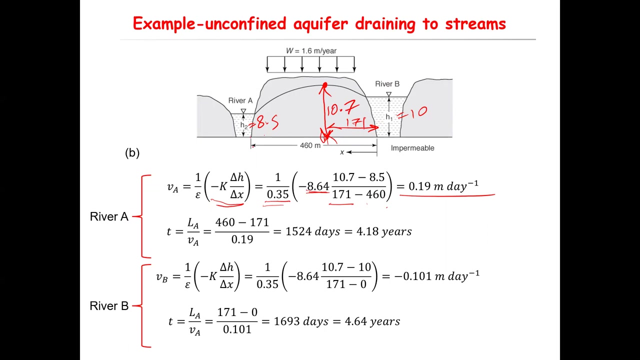 If you do the calculation, you'll end up with 0.19 meter per day. So that's the velocity. therefore, the travel, the arrival time or the travel time, what was the term I used? Yeah, the travel time will be equal to the distance divided by pore water velocity. and the distance here is: we know the total distance is 460 meter and this is 171 meter. therefore, this distance, LA, will be equal to 460 minus 175, divided by the velocity we just calculated, and that's the velocity. 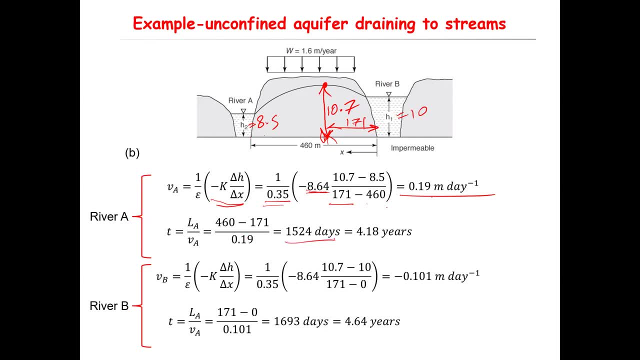 Okay, So that will be 1524 days. okay, or in other words, 4.18 years. okay, That will be the travel time from the water table divide to river A, and you can do exactly the same for river B. that is, the VB is equal to one divided by porosity, which is given times minus K. that is given times delta H over delta X. okay, 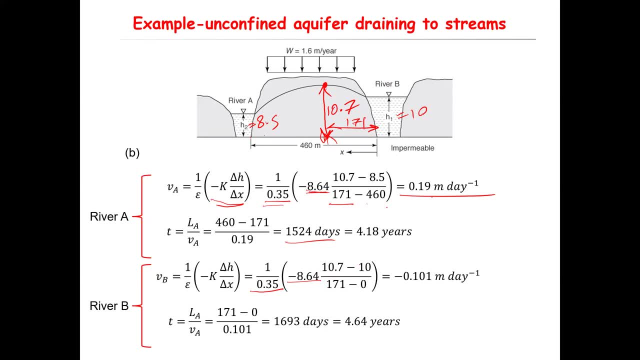 And delta H. here I have 10.7 minus the H1. here is 10, divided by 172.. That is the X of this point minus X of this point, and here is at the origin. so that is zero, okay. 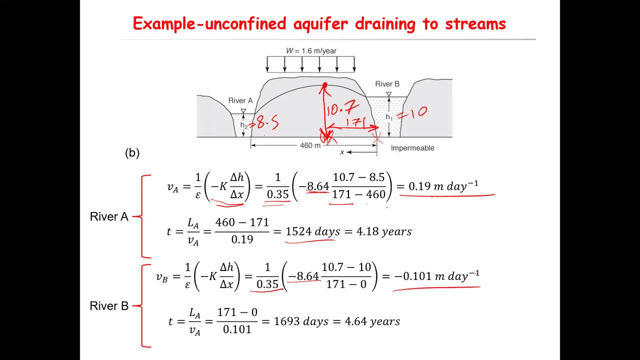 And that will be equal to minus 0.101 meter per day. You see, here in this question the X direction is considered in this way, as you can see here, right. So the minus sign, that means the flow will be in this direction, right? 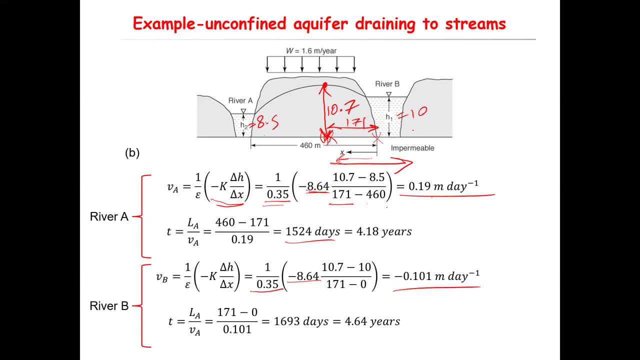 And it kind of makes sense because here you have a higher head- 10.7, than H1,, that is 10 meter, And for the travel time, again, it will be equal. So the distance divided by velocity- here we know distance- will be equal to 171 meter divided by velocity, which will be equal to 1693, okay. 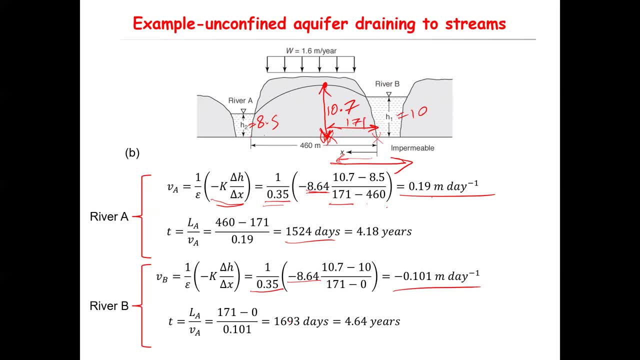 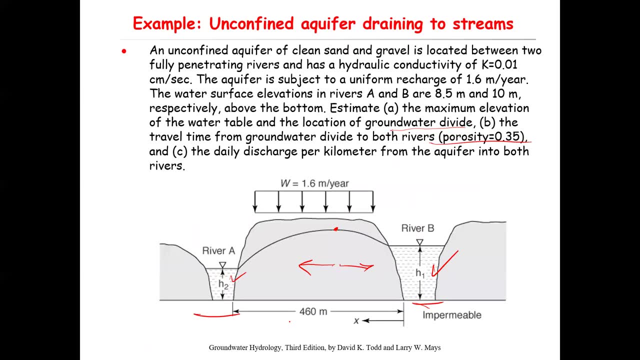 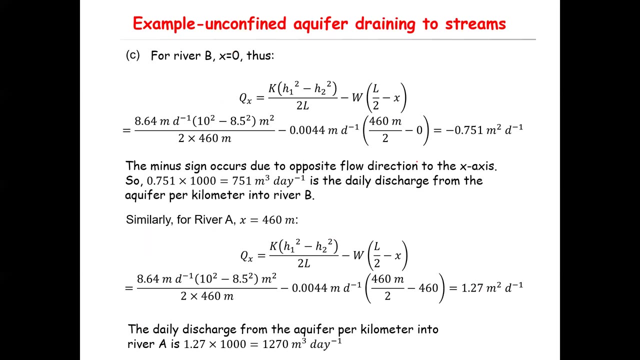 Days, which will be equal to 4.64 years. okay, And then the third part of the question. the question had three parts. The third part was the daily discharge per kilometer from the aquifer into both rivers. okay, The daily discharge from the aquifer to the rivers: okay. 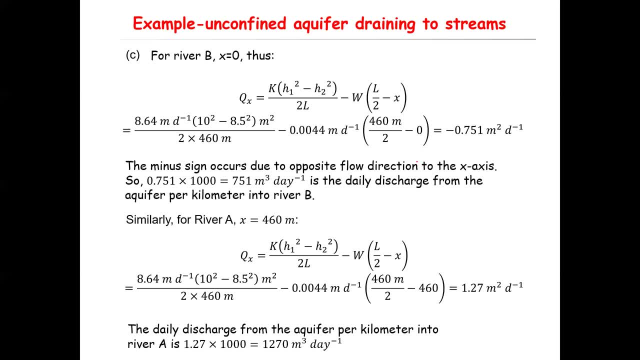 So for rivers, Okay, So river B. so river B is located at the origin. therefore, X is equal to 0.. We have this equation to calculate the discharge Again, you have all the parameters here, except you need just to put here X equal to 0. 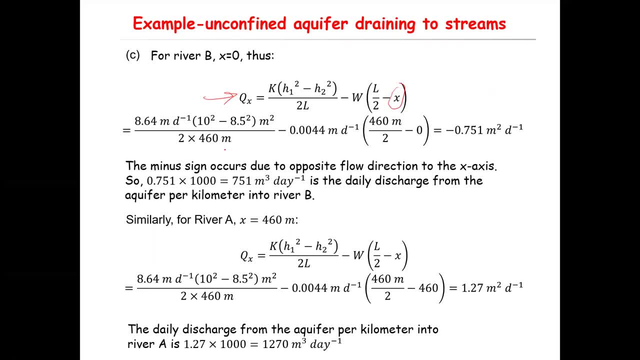 So you have the K, you have the H1,, H2, W, L and everything you put it here. that will be the QX. okay, And remember, that was the discharge per width, if you remember, or per thickness. 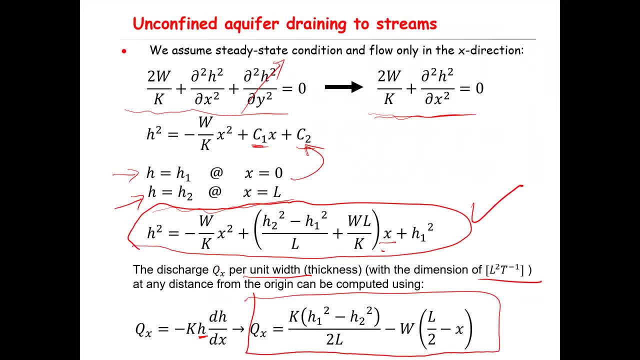 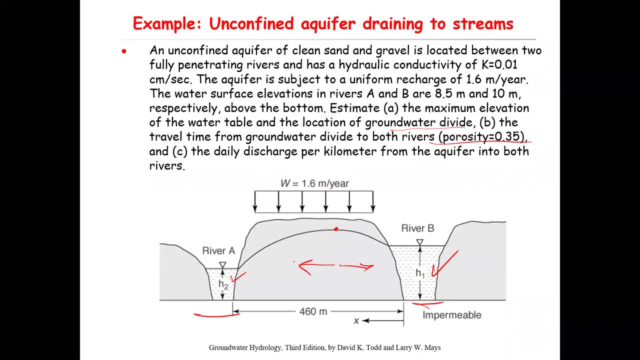 Let's go to the question. Here we call it the discharge per width, So we have the discharge QX, or this equation is QX per unit width. okay, So here in the question it says per kilometer, per kilometer. 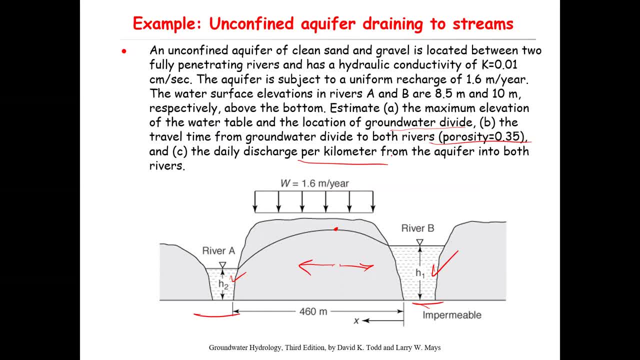 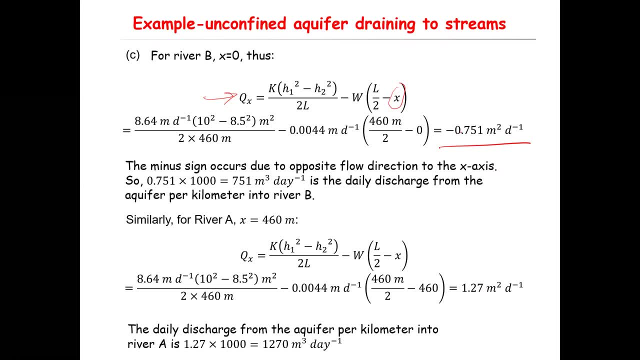 So that means that the direction perpendicular to the screen is one kilometer. So if I multiply this velocity, this discharge, basically it's not a velocity that has the unit of M2, or length squared divided by time, or it's- yeah, it's QX, the discharge per unit width. 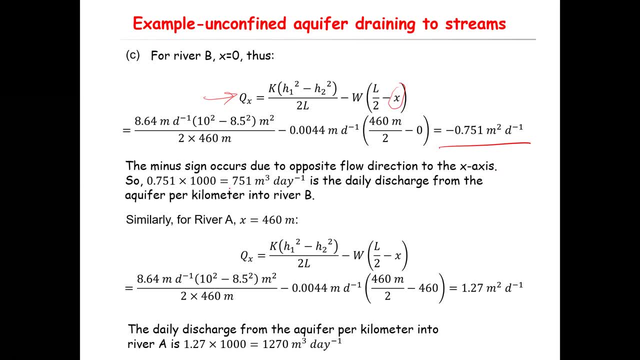 So if I multiply it by width, I multiply it by width, that is 1,000 meter, that gives me 751 cubic meter per day And that will be the daily discharge, or volumetric flux, from the aquifer to river B. okay, 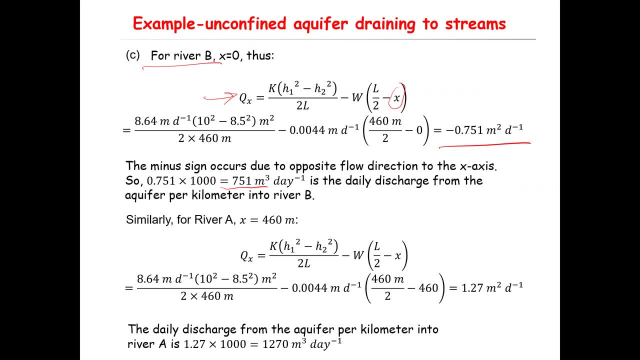 So that calculation was for river B. We can do exactly the same for river A. The only difference here is the river A. the X value is 460 meter. that's all. So again, you apply the same equation. All the parameters is given. 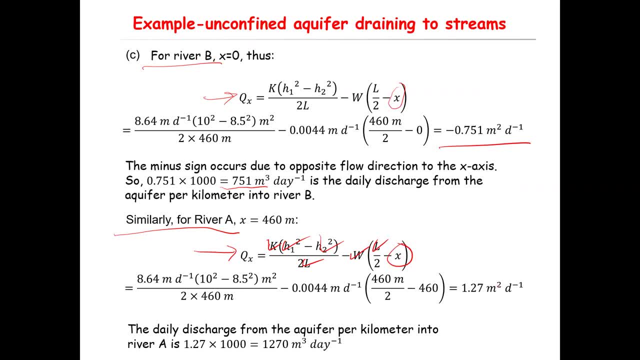 In the question, instead of X you put 460 meter, then you do the algebra, here the calculation, you end up with 1.27 square meter per day. okay, And then the daily discharge, like before, you need to multiply that by 1,000, because the question is per kilometer.